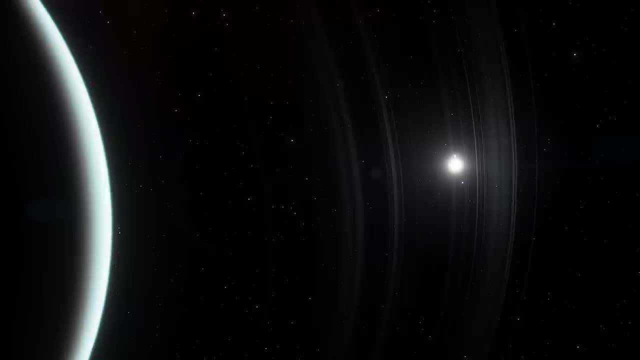 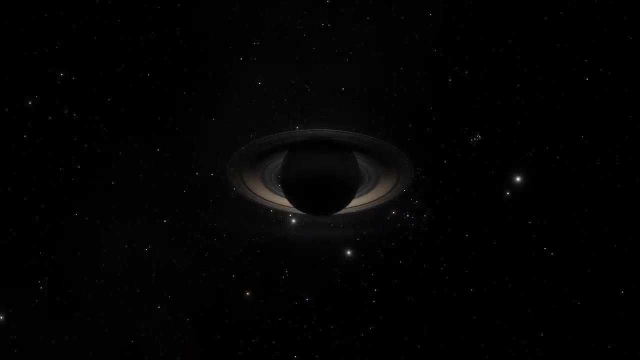 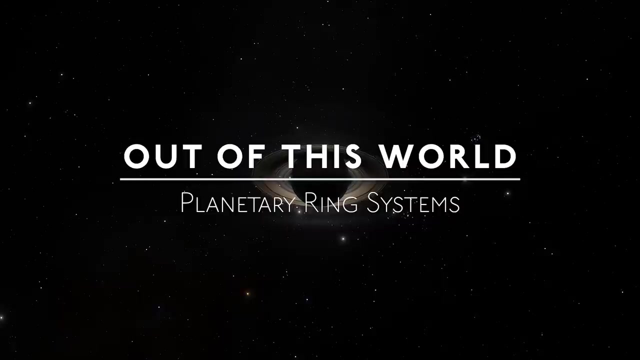 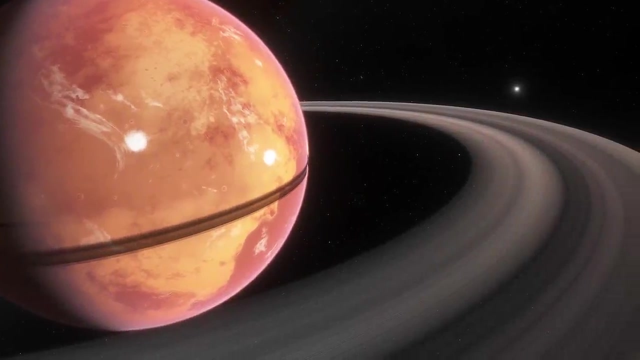 technology has led us to discover ring systems all over the solar system and elsewhere in the galaxy, And this incredible, beautiful natural phenomenon is going to be our topic today. A planetary ring system is a flat, disc-shaped collection of billions of particles and chunks. 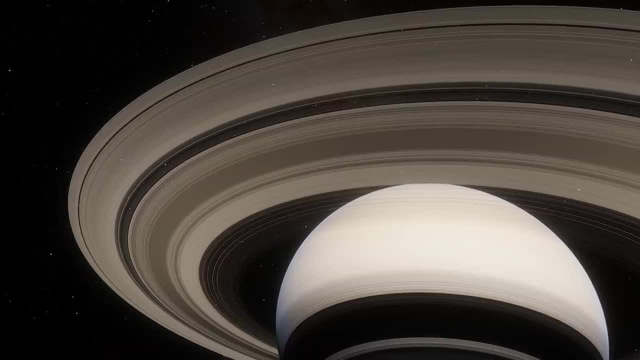 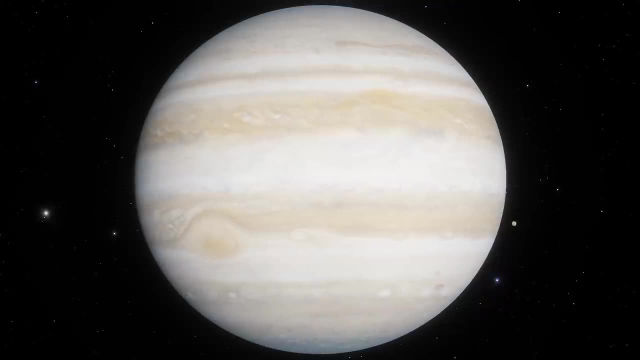 known as moonlets, which are orbiting along the ecliptic plane of a planet. As planets rotate, the force exerted causes them to bulge slightly at their equators. This causes them to move, and this defines an equatorial plane for the planet along which satellite material 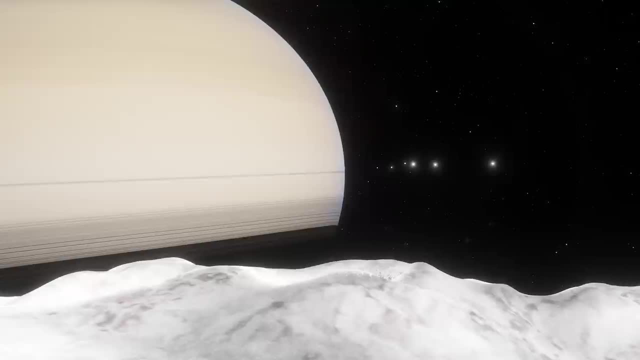 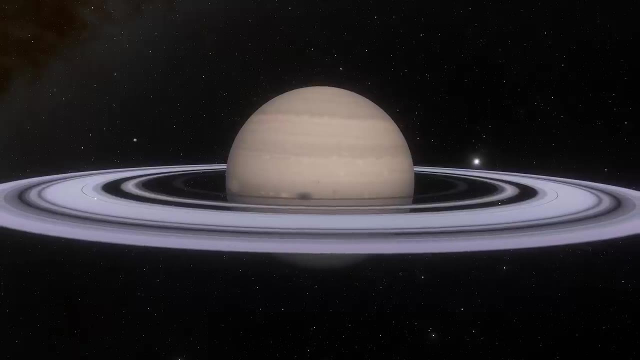 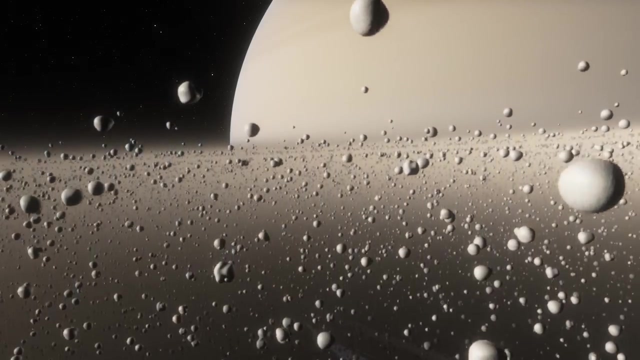 tends to orbit. As such, the moonlets within a ring system experience only very minor vertical motion. Rings can be millions of kilometres in diameter, yet only a few dozen metres thick. The structure of these systems is impressively complex and sculpted by gravity both from 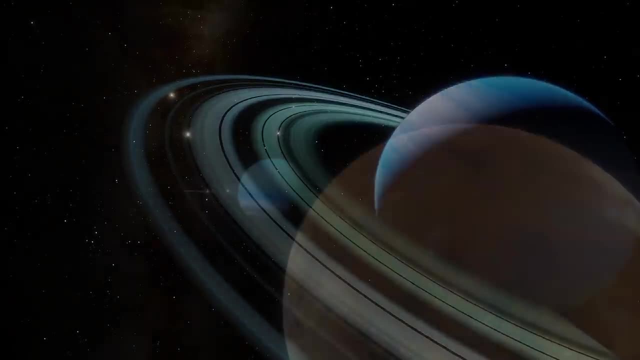 the host planet and from the moons elsewhere in the galaxy. The structure of these systems is impressively complex and sculpted by gravity both from the host planet and from the moons elsewhere in the galaxy Within the vicinity of a ring system. the tidal stresses from the parent planet are 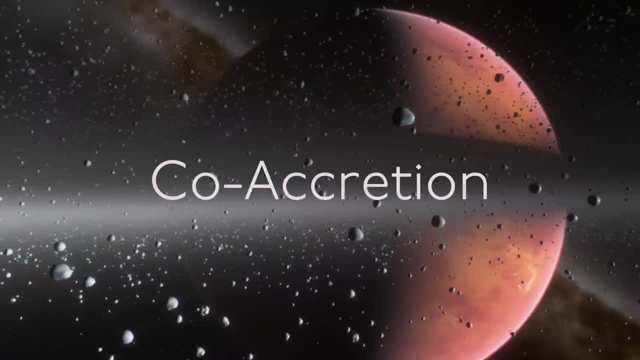 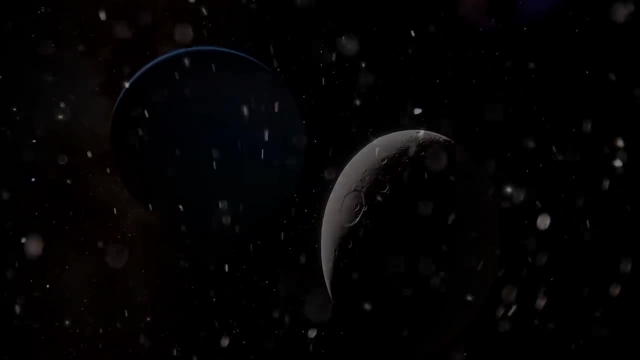 too strong for the moon-forming process of co-accretion to occur, and so, rather than collecting to form new moons, the moonlets within a ring system are kept in a fine state. They can be anywhere from molecule-sized to house-sized, but they don't get any larger. 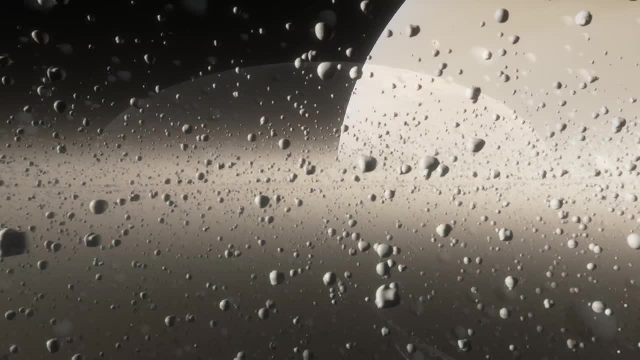 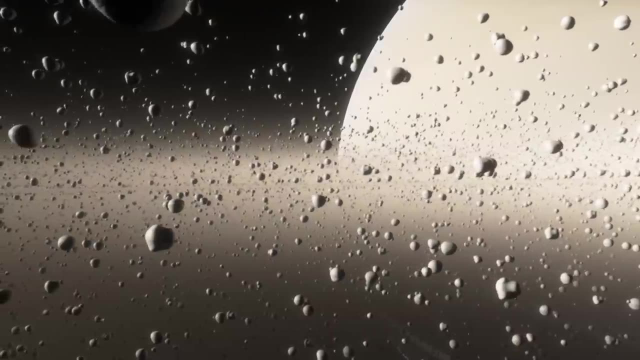 than that. Each individual moonlet in a ring system can be thought of as a single particle, becoming a tiny moon and taking its own path around the planet. Moonlets on the inner part of the ring system complete orbits quicker than those on the outside, which causes one. 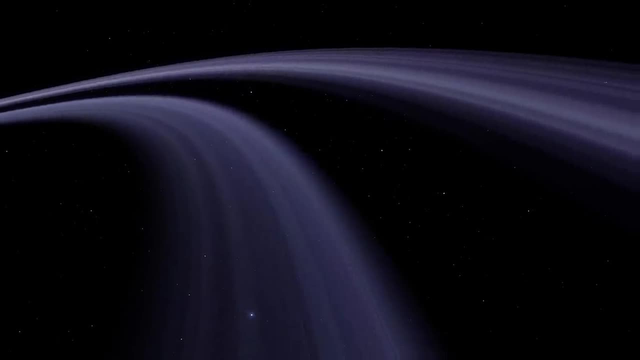 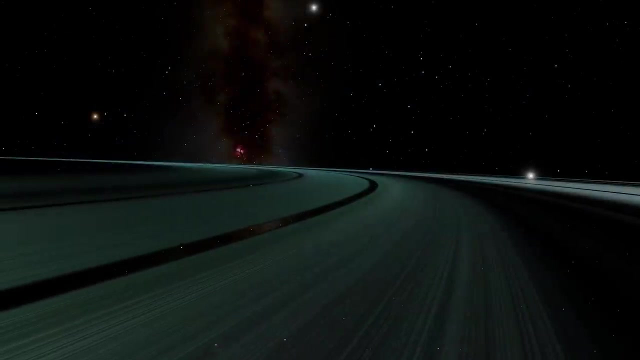 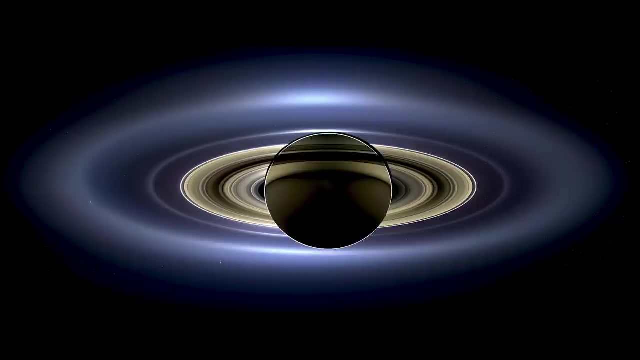 disk to fragment into several narrower, denser ringlets, And both are made up of dozens of even smaller ribbon-like lanes of particles. Of course, Saturn's rings are by far the most fantastic and indeed the most studied in the solar system. But do you have anyisu vegg ins? 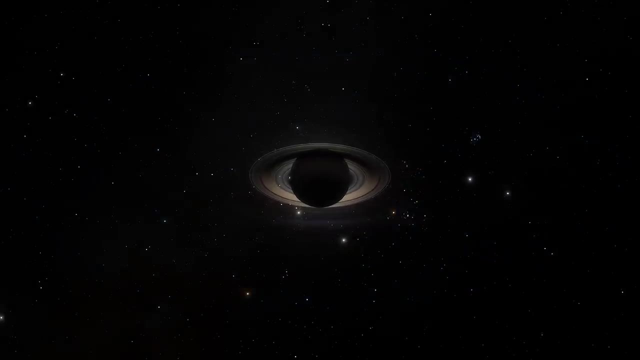 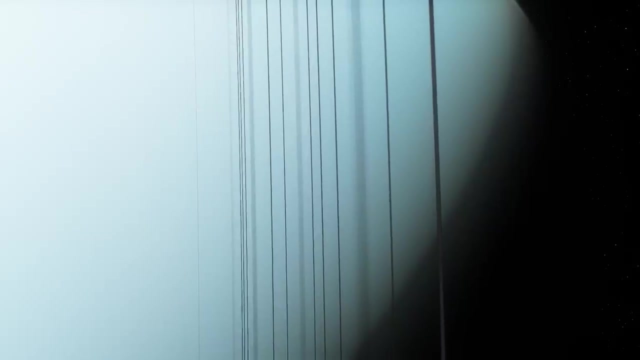 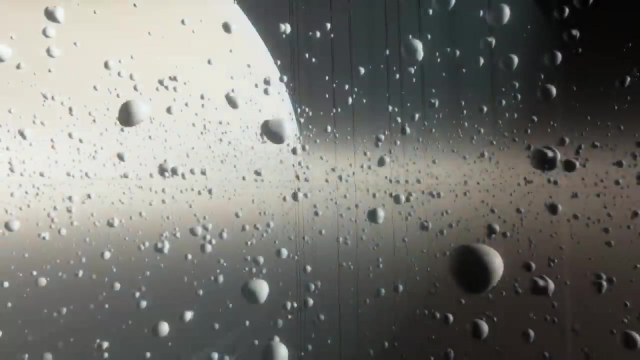 system, But the Voyager spacecraft in the 1980s revealed to us that each of the four gas giants houses a ring system, but each varies wildly in its composition, arrangement and overall substantiality. The rings of Saturn are made up of highly reflective water ice. 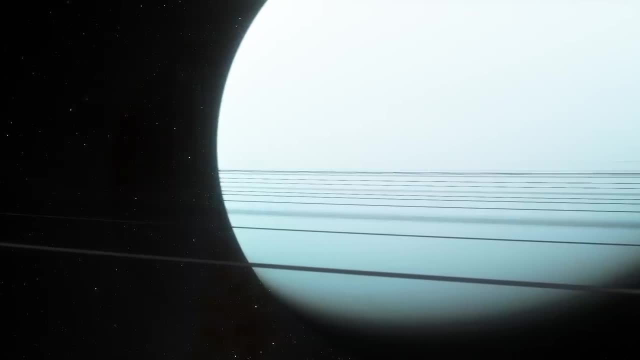 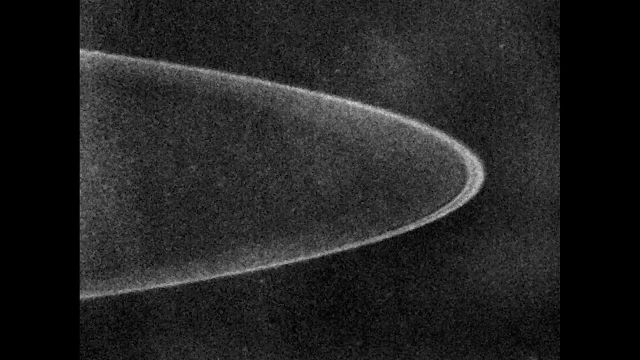 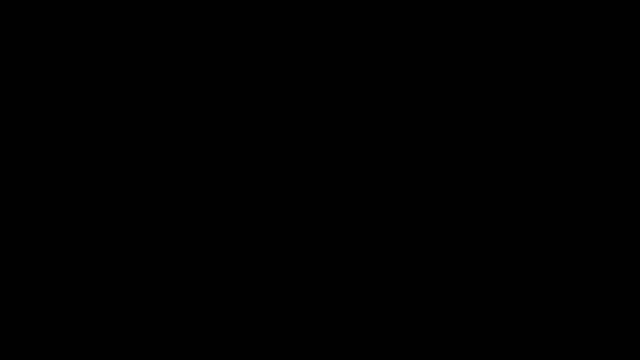 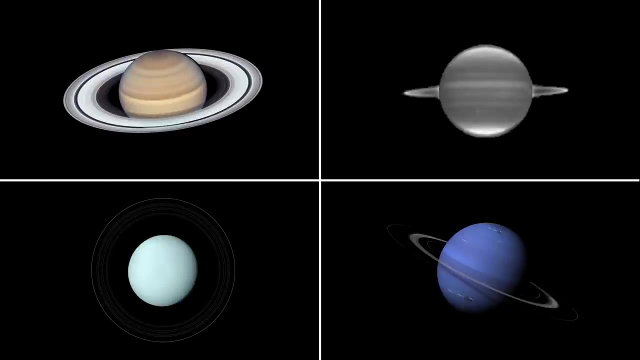 whereas the rings of Uranus are made from organic material as dark as charcoal, Jupiter's enormous yet faint ring system is composed mostly of ancient dust, and Neptune's rings are a mixture of dust and shredded rocks floating around in the darkness. We don't fully understand the underlying mechanisms that connect these ring systems. 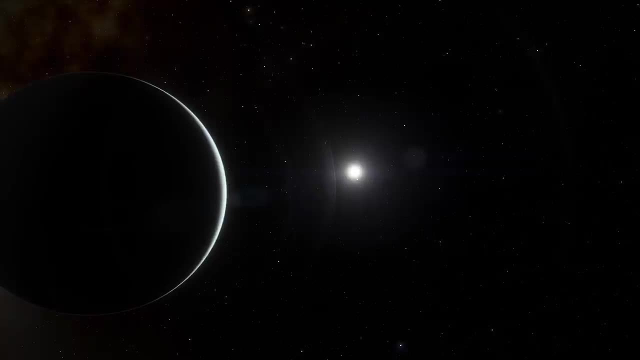 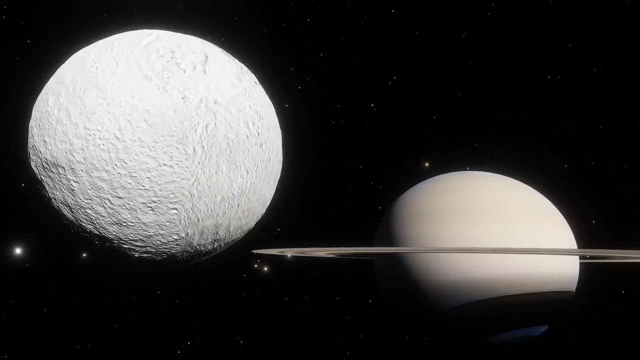 and it's likely that each has a different story to tell. But one thing we do know is that ring systems almost certainly need moons to be both created and sustained. So let's take a closer look at each of these rings and see if there's anything. 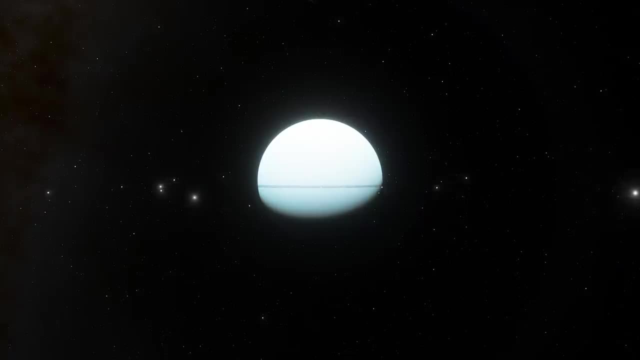 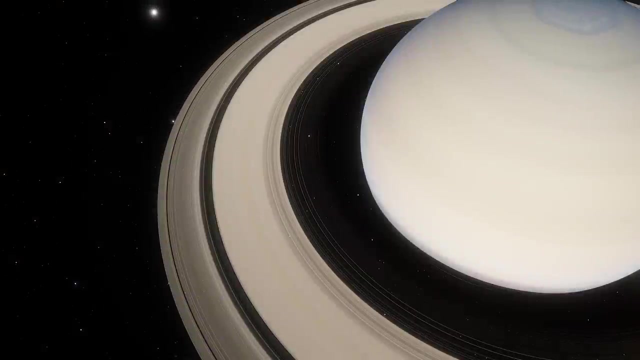 we can do about it. If it were not for the tidal interactions and orbital resonances of the gas giants moons, much of the material we see in their ring systems would be flung out into space. Therefore, it may be the case that ring systems exist wherever there are moons to be found, Not 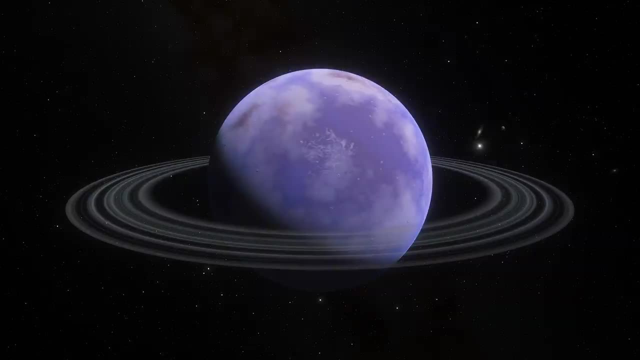 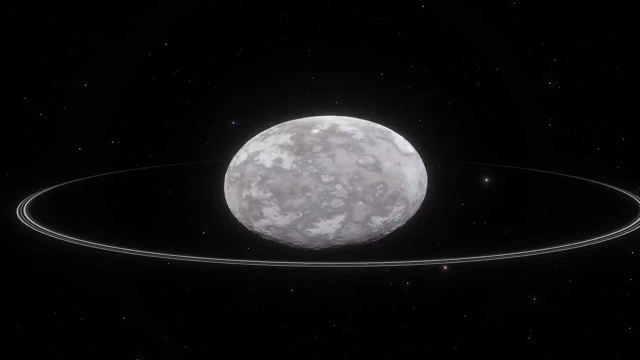 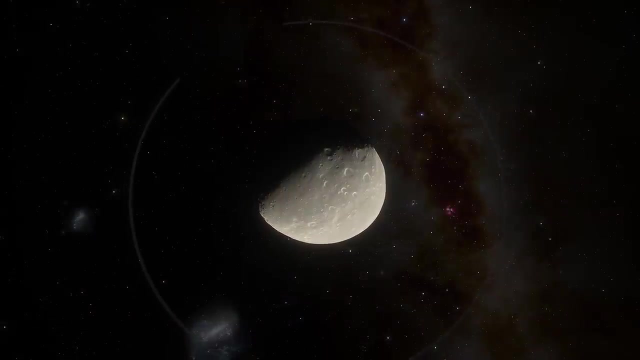 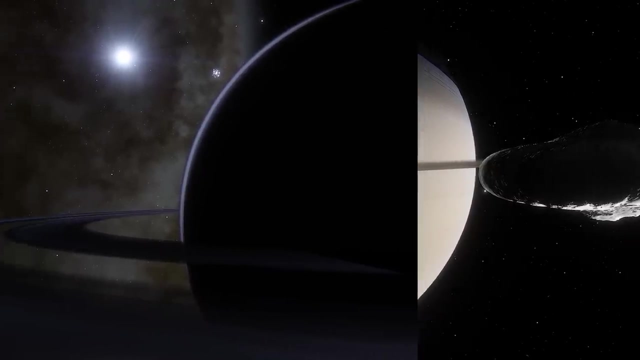 just around gas giants, but around earth-sized worlds, brown dwarfs, infant stars, dwarf planets and even moons themselves. Any world can have a ring system if the prerequisites are right. But what are those prerequisites? Well, there are two main hypotheses for how ring systems come to be formed. The first hypothesis 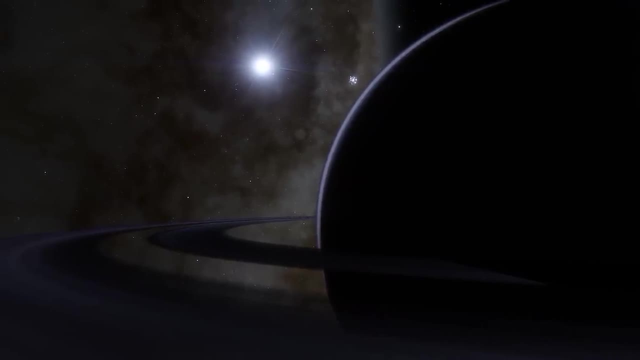 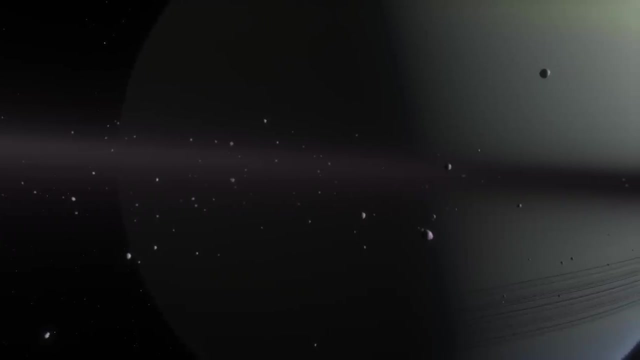 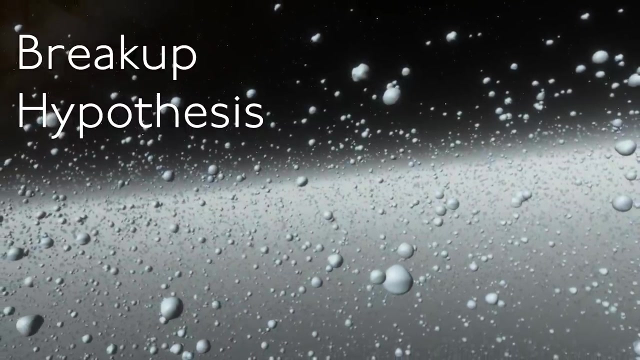 states that ring systems can be formed during the birth of the parent planet- from leftover dust and material which is too close to the planet's surface to be able to coalesce into a moon. The second is the break-up hypothesis, which states that rings are the result of shattered moons which either got too close to their 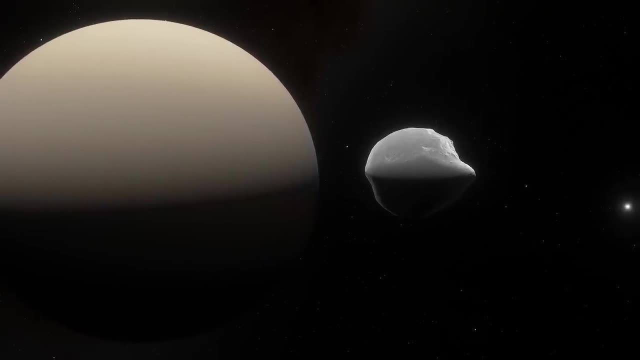 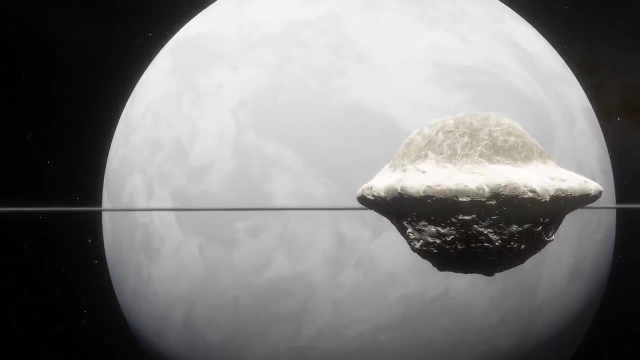 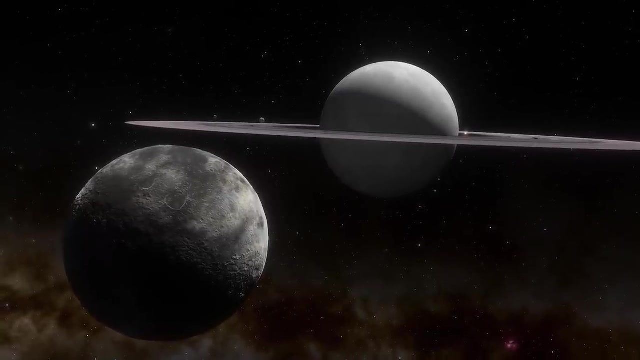 parent planet or were involved in a collision which shredded them down into chunks which dissolved. In both cases, the gravity of the host planet plays a key role. Where two celestial bodies of differing masses exist, for example a large planet and a small moon, there comes. 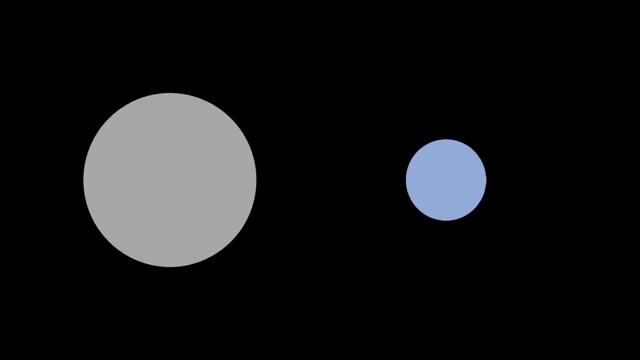 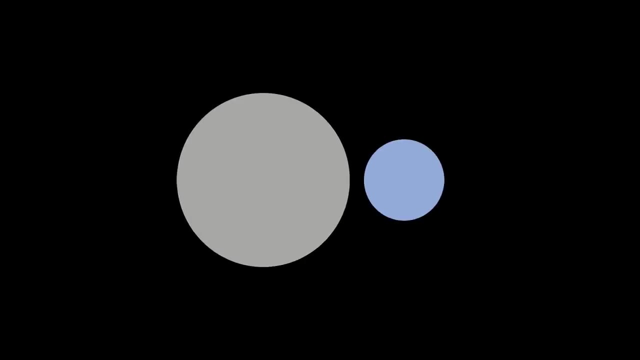 a distance between the two objects, known as the Roche Limit, where the tidal stresses from the larger body will exceed the smaller body's ability to keep itself held together, causing the smaller body to be pulled apart and dissolved into moonlets. This material, 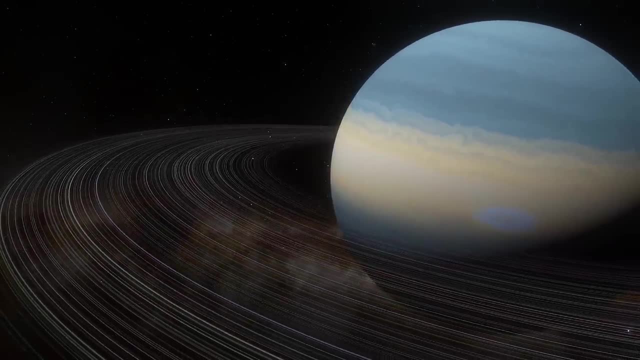 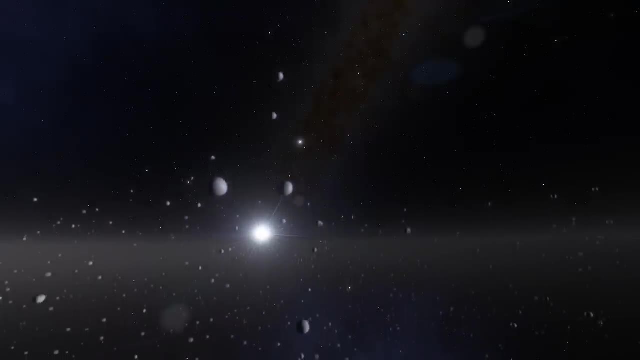 then collects along the common plane of the planet into a disk comprised of tiny individual chunks, each with a much lower mass than the moon that came before it, And because they lie within the Roche Limit of their host any time these moonlets come together to form. 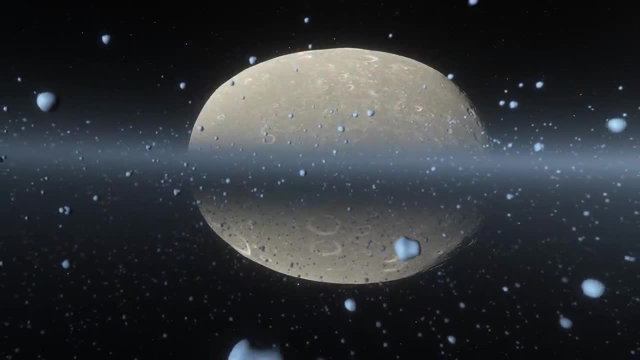 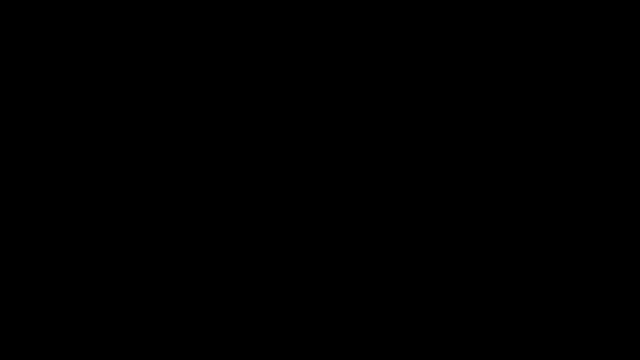 anything larger than house size or the size of the moon itself. the two object will be sized boulders. tidal forces will break it back down. Co-accretion becomes impossible, Of course. the more massive an object is, the stronger its ability will be to keep itself. 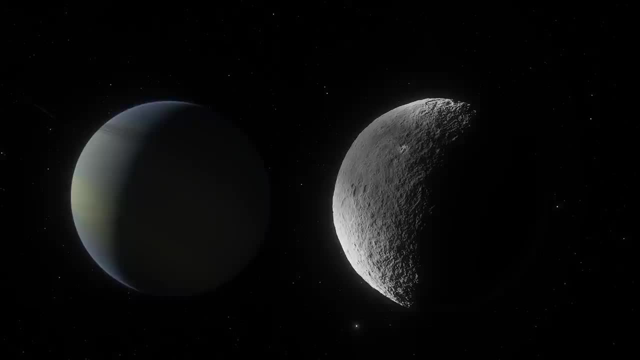 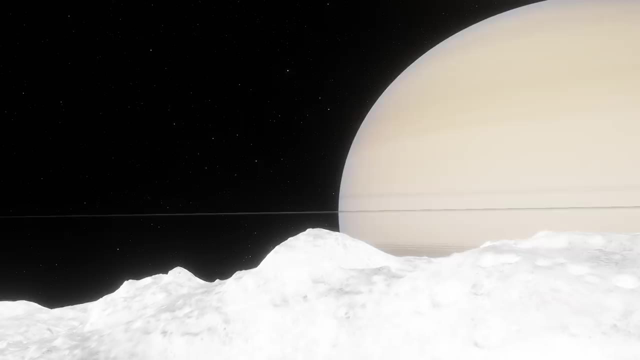 held together through gravity, And so that's why we see moons orbiting in around and between ringlets without breaking up- their gravity is much stronger than that of the moonlit chunks, and so they would need to get a lot closer to the parent planet before they succumbed. 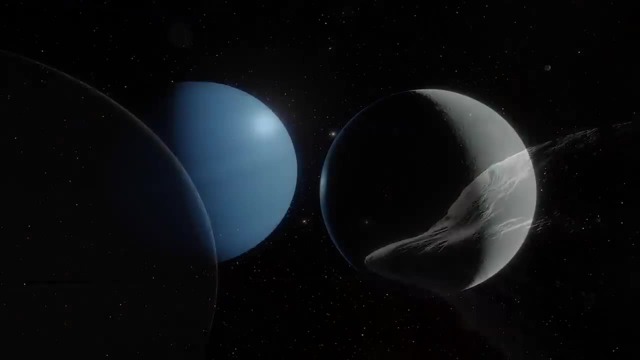 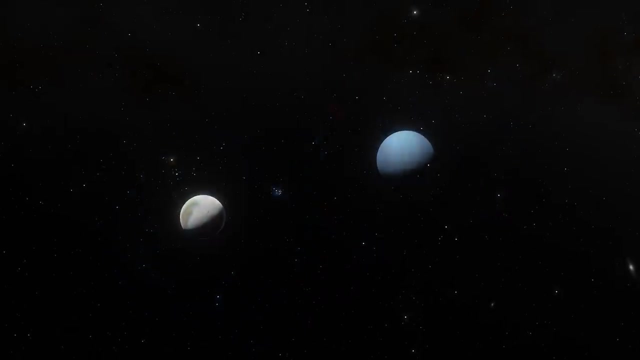 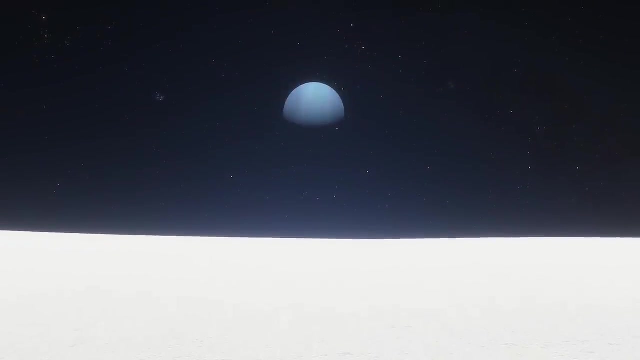 to tidal forces. Such a fate awaits Neptune's moon of Triton in about 3.5 billion years. Triton's decelerating orbit is bringing it ever closer to Neptune and it will eventually draw so close that it will be ripped apart by tidal forces forming bright and brilliant. 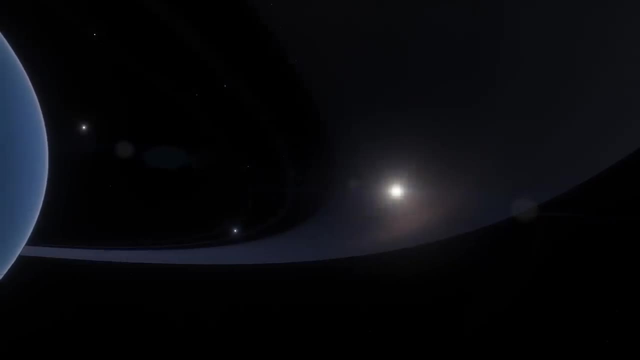 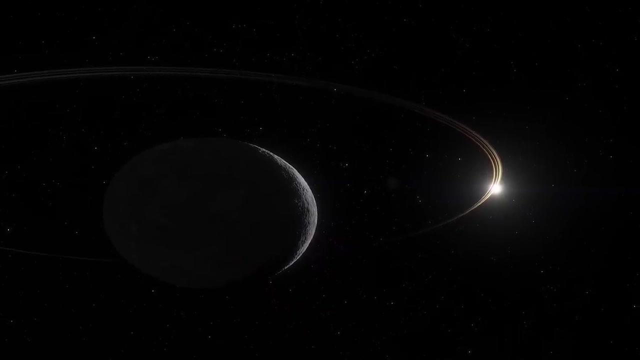 new icy rings around the planet. This is how we think Saturn is going to look like. This is how we think Saturn is going to look like. This is how we think Saturn is going to look like. Saturn, Neptune, Uranus and the dwarf planet Haumea got their rings. As for Jupiter, well, 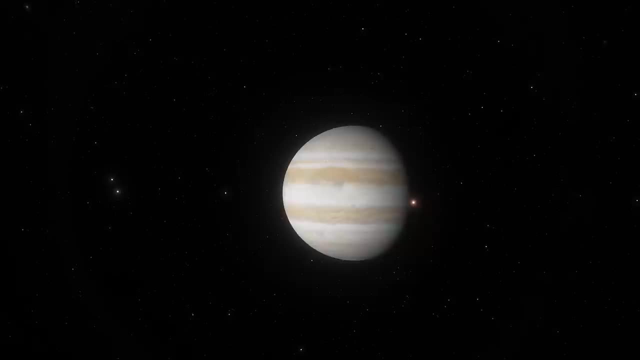 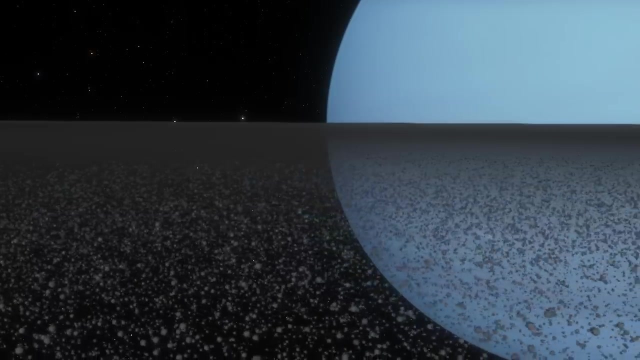 they are more likely to be primordial in origin, and so it would seem that we have evidence of both ring-forming hypotheses playing out right here in our own backyard. But of course, Jupiter's ancient and tenuous ring system is nothing when compared to that. 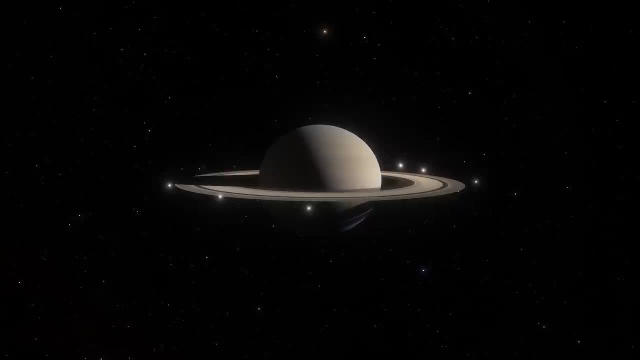 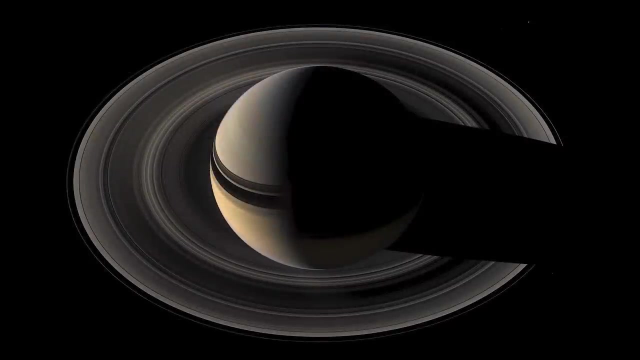 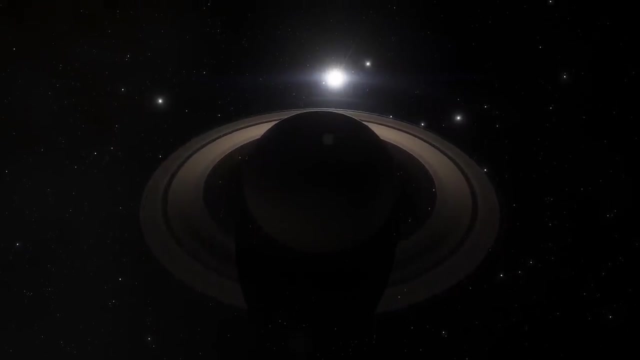 of its sibling. In fact, nothing quite compares to the rings of Saturn. They are by far the planet's most distinguished feature and indeed one of the most breathtaking sights in the solar system, stretching out into space and gleaming under the light of. 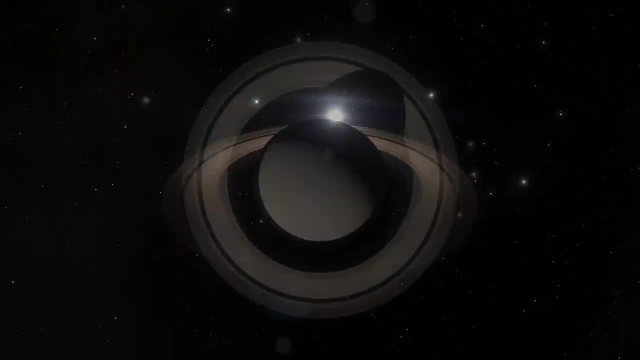 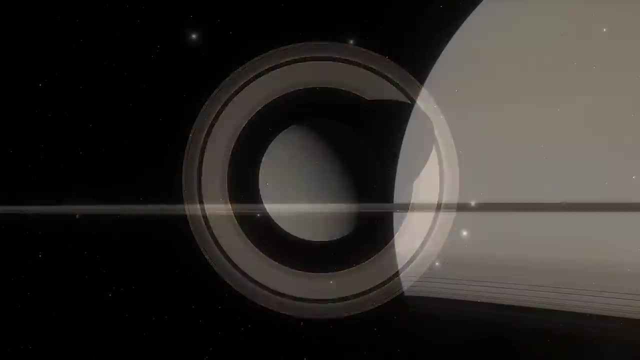 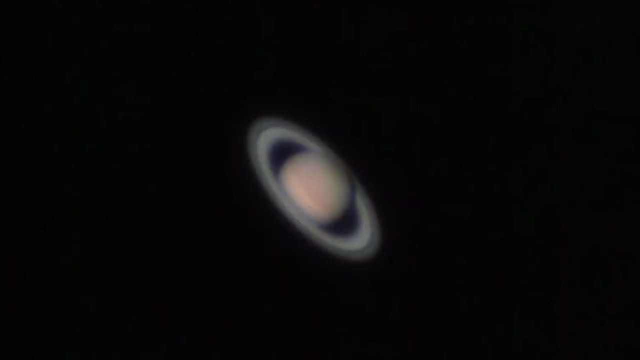 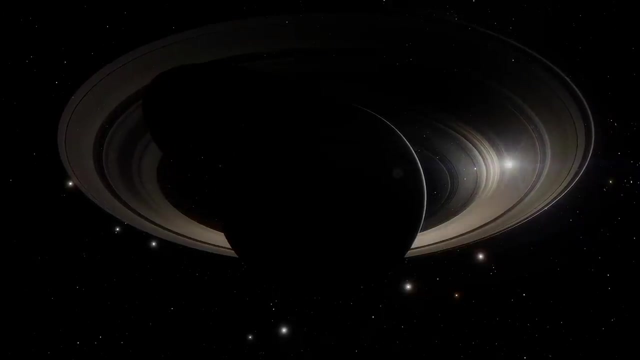 the sun. The rings extend over 140,000km, more than twice that of Saturn itself, yet they are only around 20 meters thick on average. The striking, shining protuberances they give Saturn stuck out to early astronomers where other ring systems remained hidden, As we mentioned at the start. 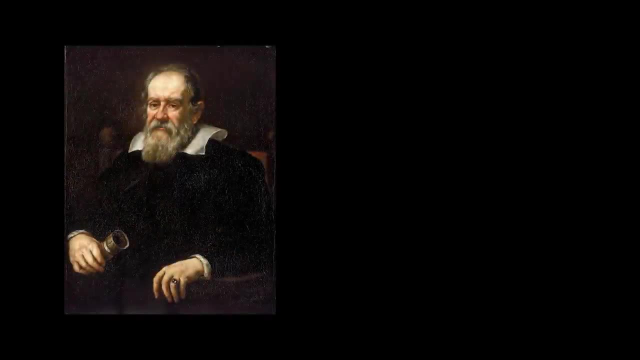 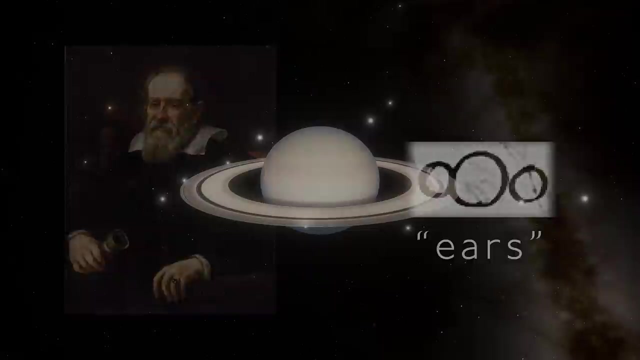 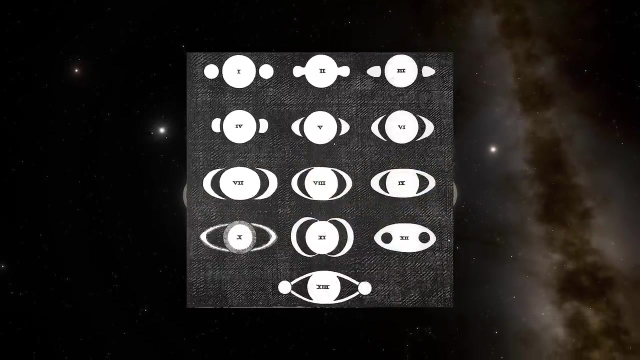 it was Galileo who first noticed Saturn's rings, but he was unable to accurately describe them, initially, mistaking them for handles or ears of the large planet. It took another five decades for us to realise that the rings are not part of the planet itself and another. 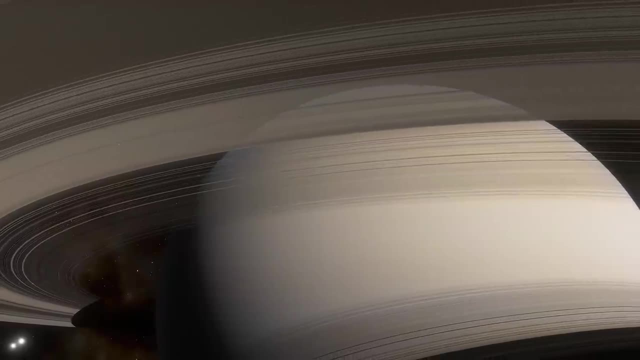 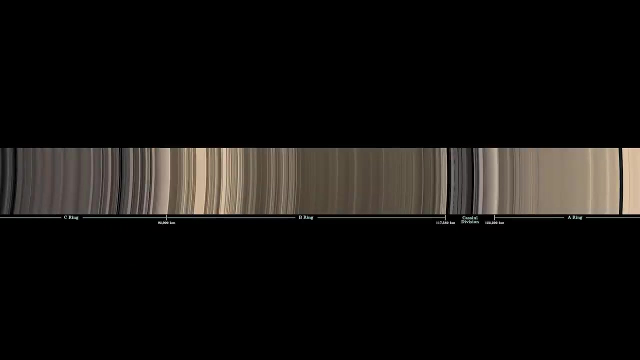 200 years to accept that the rings themselves are not a solid structure, Though they appear as one from the point of view of the Earth. the system is separated into several subdivisions, labelled A through G, based on the order in which they were identified. 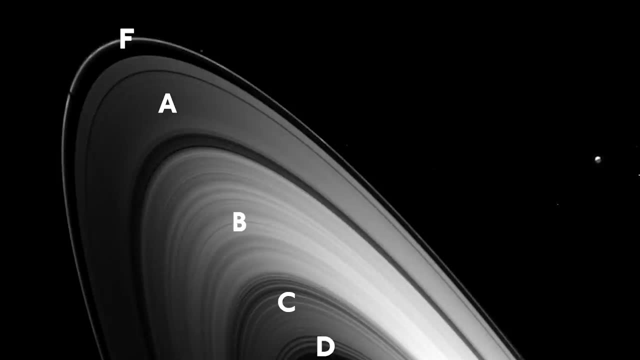 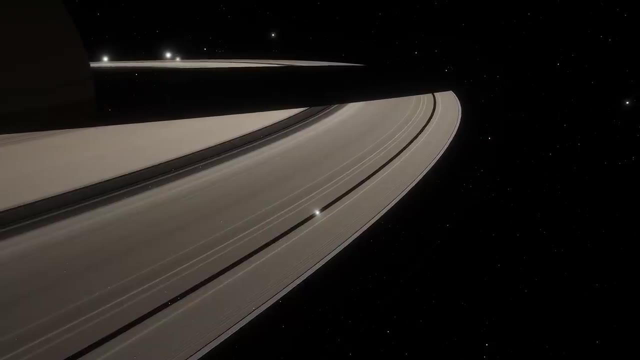 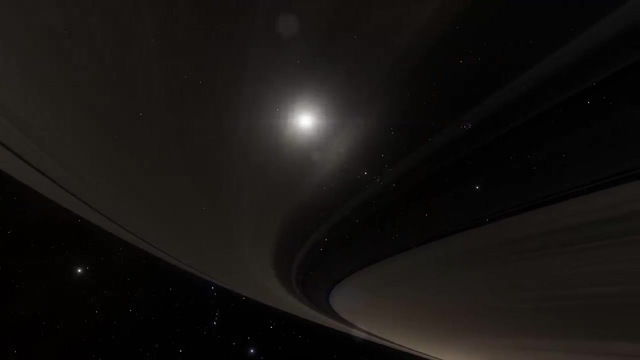 The rings D, C, B, A and F lie on the inside, with E and G further out, separated by gaps and trails through which Saturn's moons have passed and cleared out material. These seven main rings are themselves composed of multiple rings, each of which has its own. 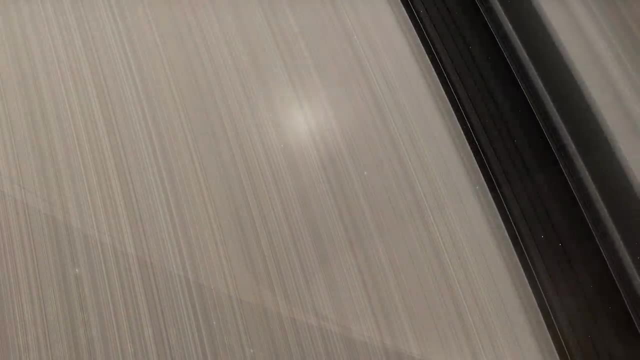 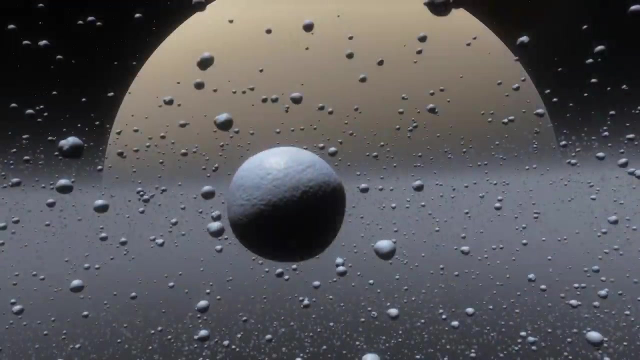 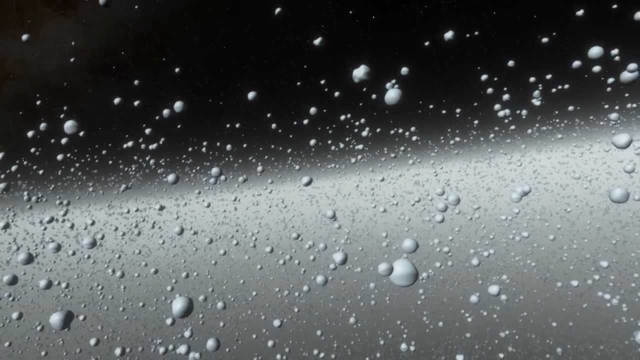 much smaller ringlets- there may be as many as 500 to 1000 of them in total. From the very inside, the rings would appear much like floating in a cloud of snowballs and snowflakes, with icy dust and hailstones streaming around in between, While the Cassini spacecraft didn't. 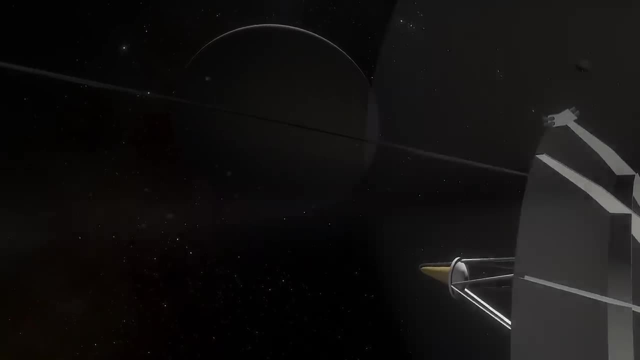 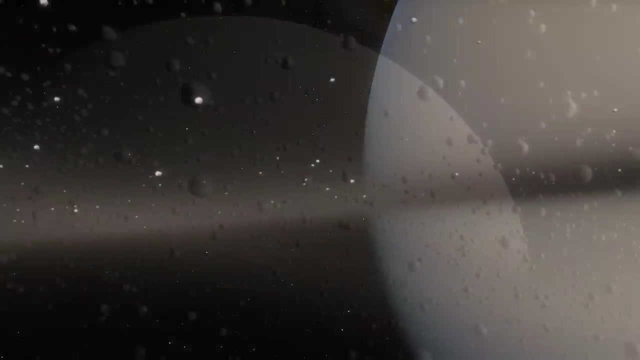 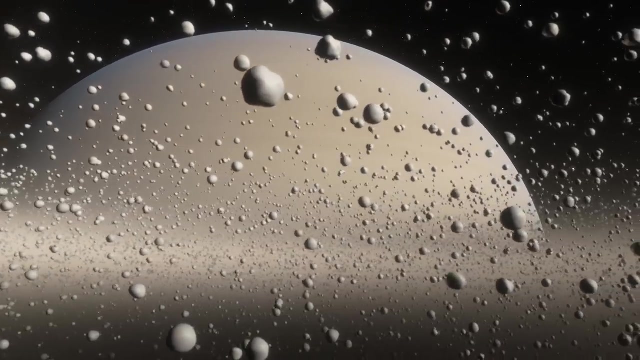 manage to get this close, it nonetheless revealed activity within the rings on wildly differing timescales- from months and years to just a matter of days. As moonlit chunks come together and interact, reverberations cascade through their surroundings like gravitational ripples in a lake of ice, Given that the rings are so water-ice rich. 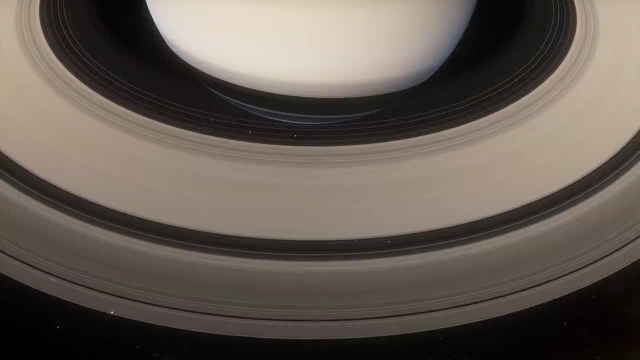 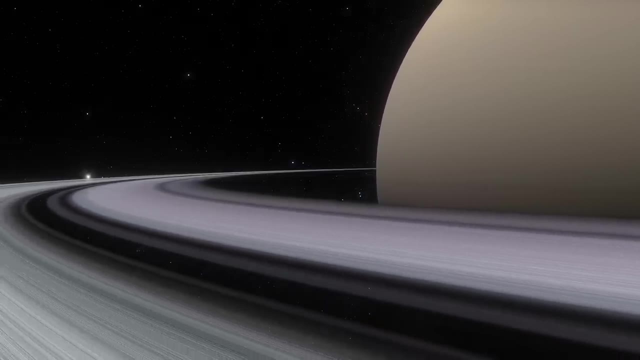 it's very unlikely that they are primordial in origin. If they had formed from the protoplanetary dust which gave rise to Saturn, then they would not be nearly this reflective, But instead they shine due to their high water-ice content. 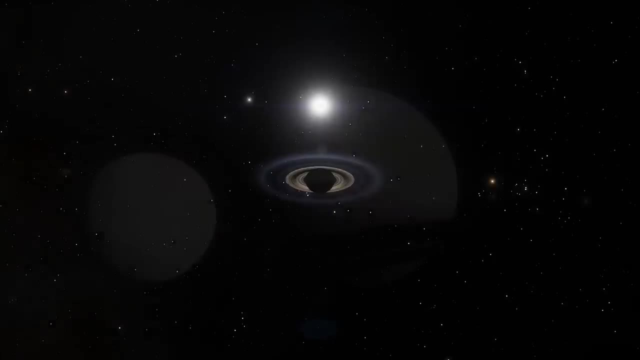 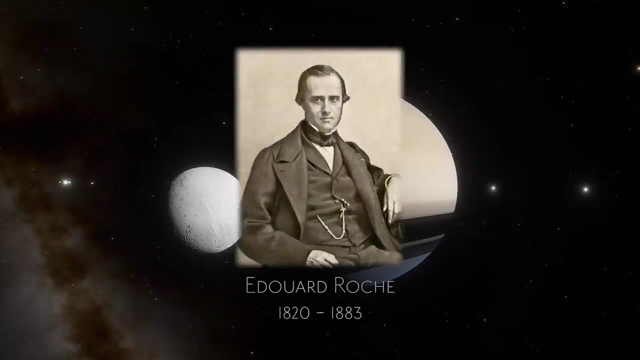 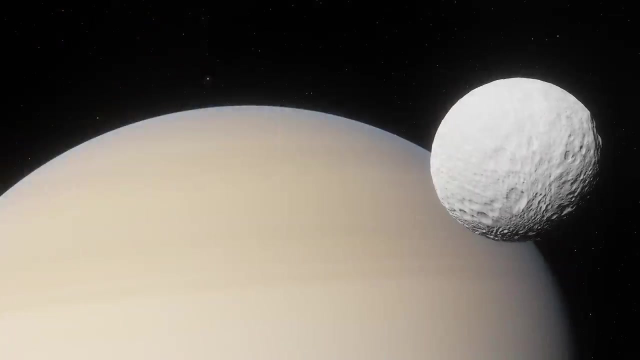 This suggests that the rings were formed through the break-up of one of Saturn's icy moons- a possibility proposed by none other than the architect of the Roche Limit, Eduard Roche, in 1849.. It is thought that a moon, perhaps similar to Titan or smaller, may have gotten too close. to Saturn, Rather than the whole body dissolving completely. the ill-fated moon would have had its water-ice mantle and crust ripped off by tidal stresses, leaving only the surface of the dense rocky core intact. The dead core of this moon would have fallen straight. 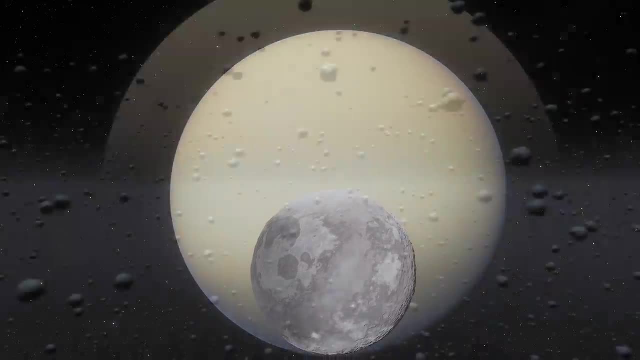 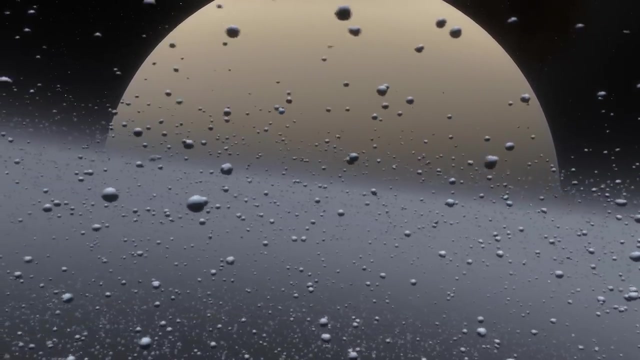 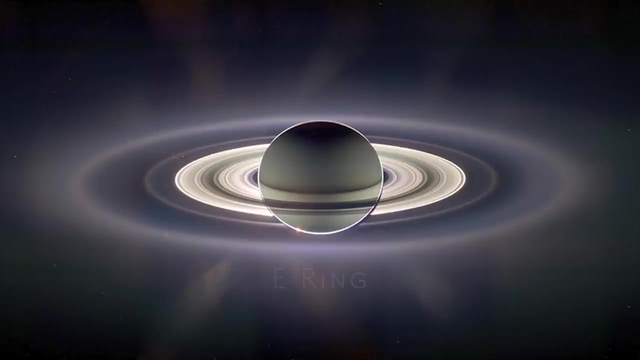 into the gas giant with the residue of its icy exterior, collecting into the ring system of particles that we see today surviving over billions of years. as one of the solar system's great wonders, These rings, in particular the E-Ring, also receive a little extra assistance in staying. 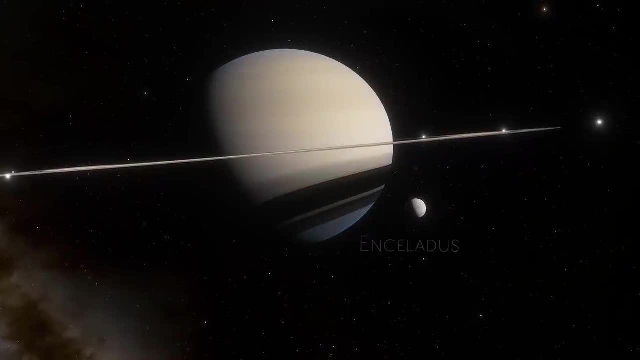 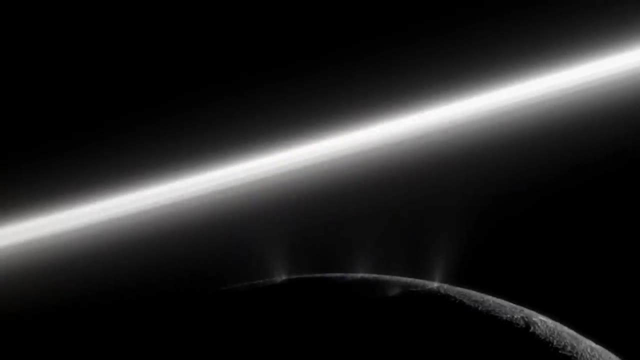 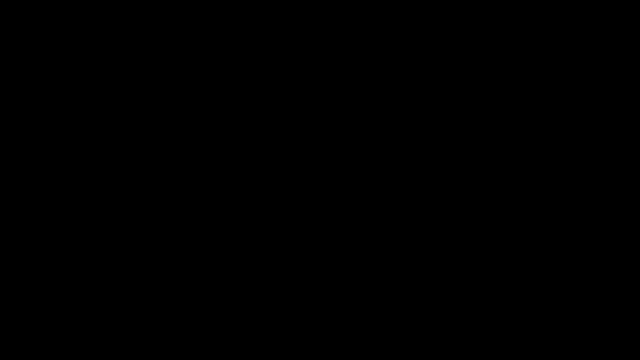 so bright thanks to Saturn's cryonics, Saturn's cryo-volcanic moon of Enceladus, which erupts plumes of liquid water and water-ice into space, feeding the E-Ring and providing a fresh source of icy material. 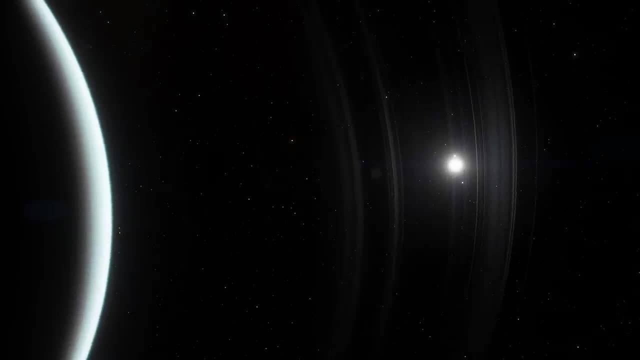 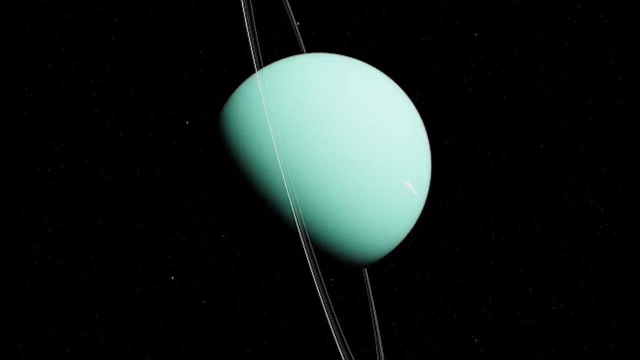 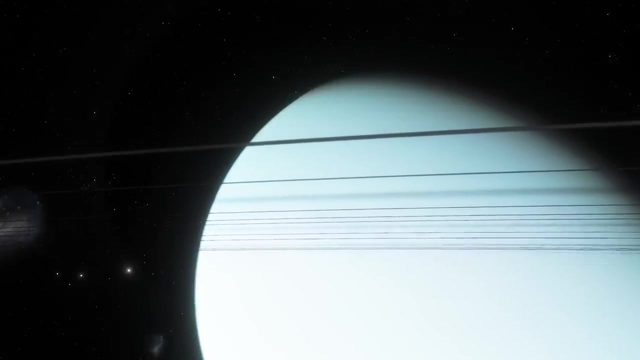 While not as bright, striking or complex as those of Saturn, the ring system surrounding Uranus is still both captivating and mysterious. Unlike Saturn, Uranus' rings do not have much shine- quite the opposite, in fact: Its moonlets constitute dark and unreflective. 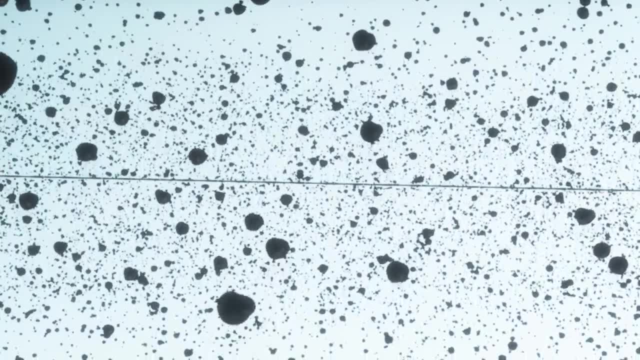 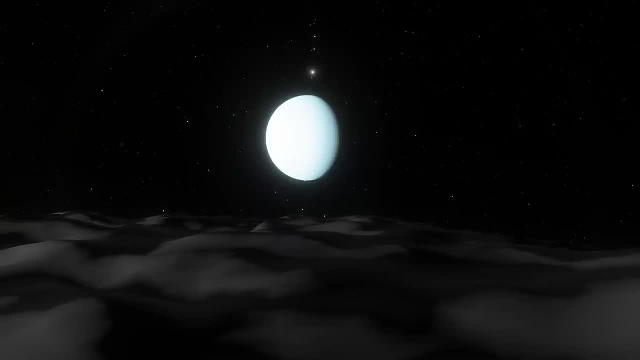 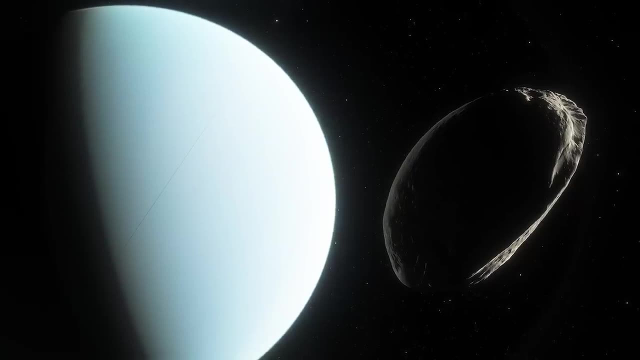 rocks between 20 centimetres and 20 metres in diameter, suggesting that they are made of organic materials such as hydrocarbons, the likes of which are more prevalent in the outer solar system. In addition, Uranus' ten closest satellites appear to share compositional characteristics. 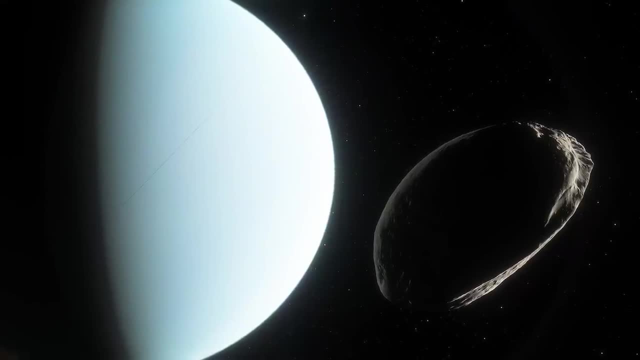 with the ring material, suggesting that this ring system is more likely to be a source of oxygen, which is why it is called the E-Ring. In addition, Uranus' ten closest satellites appear to share compositional characteristics with the ring material, suggesting that this ring system is more likely to be a source of oxygen. which is why it is called the E-Ring. The E-Ring may also have been formed by a shattered moon, but a much smaller moon and not one made of water ice. Uranus' ring system is composed of 11 fine ringlets, much thinner than those of Saturn. 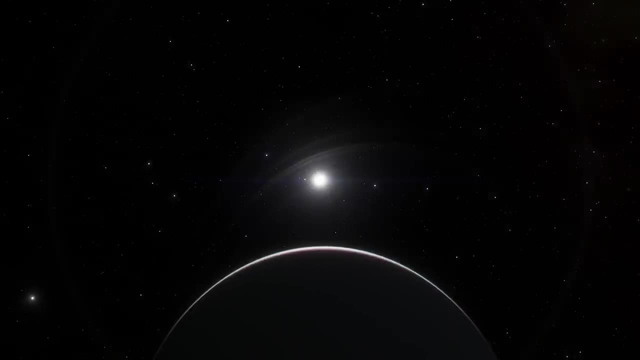 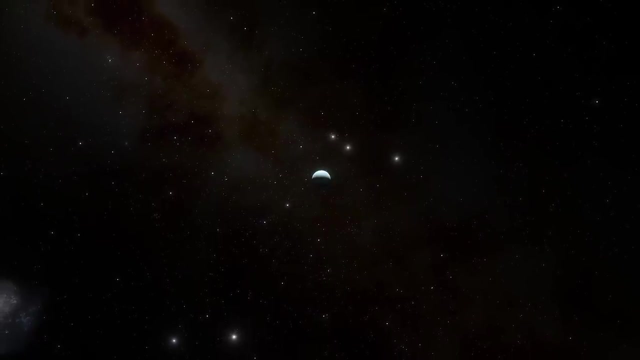 making them even trickier to spot Due to their low reflectivity. we didn't know that these rings existed for the longest time. It was only in 1977, when Uranus passed in front of a star that was under observation, that the ring system was formed. 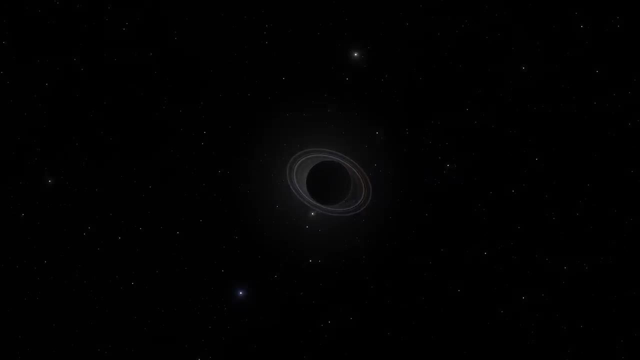 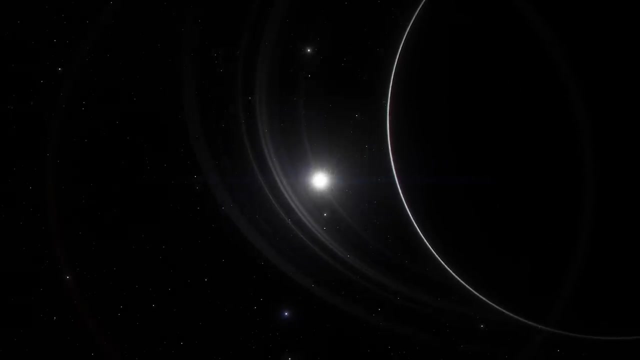 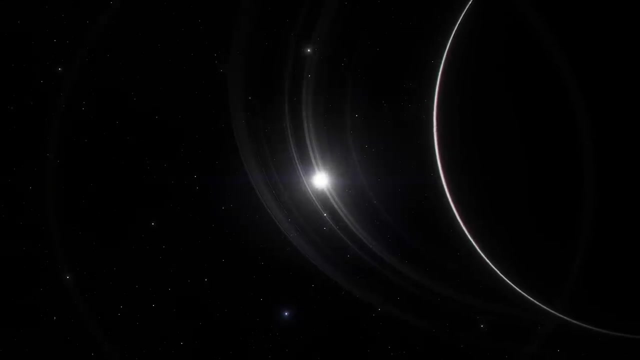 This transit allowed us to count 9 rings back then, and two more were discovered in 1986, when we first saw the planet up close through Voyager. The most substantial ringlet is the Epsilon Ring, about 100 kilometres wide and no more. 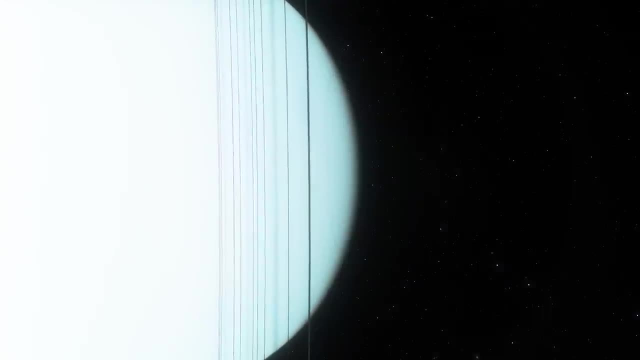 than 100 metres thick, orbiting at twice the distance of Uranus' outer edge, well within the planet's Roche limit. Uranus' outer edge is about 100 kilometres wide and about 100 metres thick, orbiting at twice the distance of Uranus' outer edge, well within the planet's Roche limit. 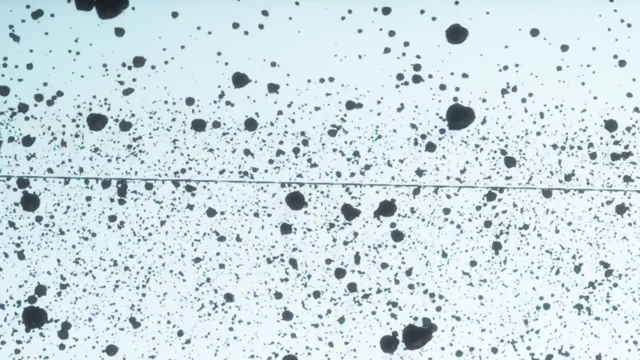 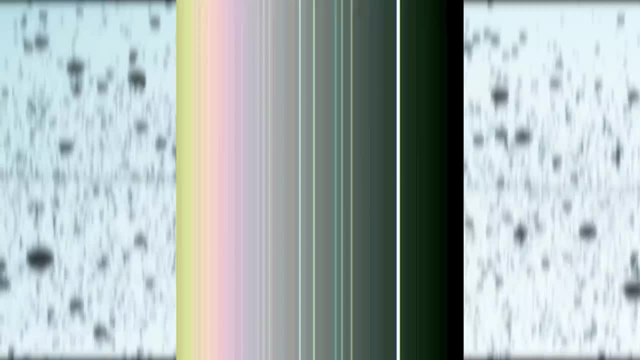 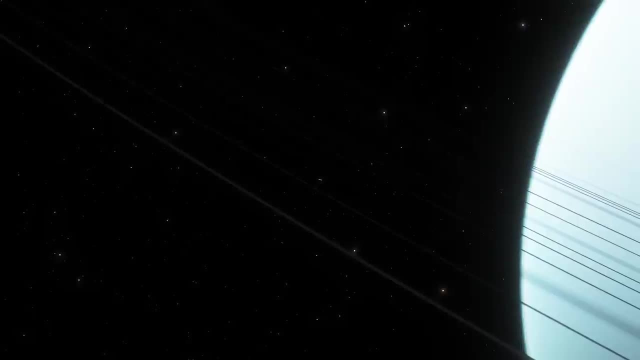 The Epsilon Ring probably contains more than 10 times the material of the other 10 rings put together. Most of the other rings are no more than around 10 kilometres wide, and this rigorously fine structure suggests that something is keeping the ringlets bound tightly. 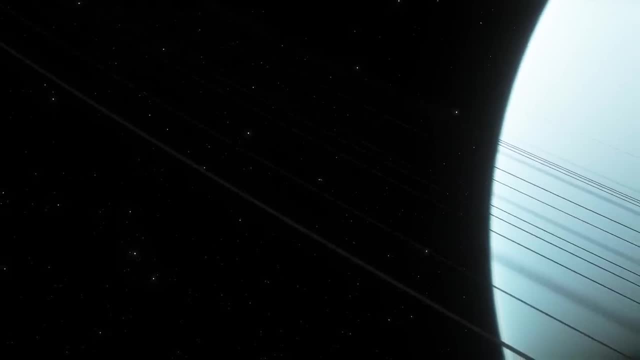 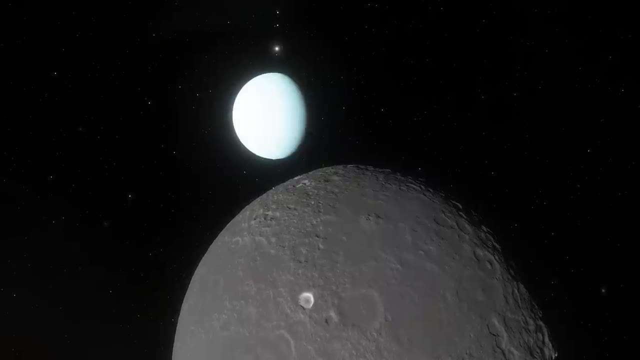 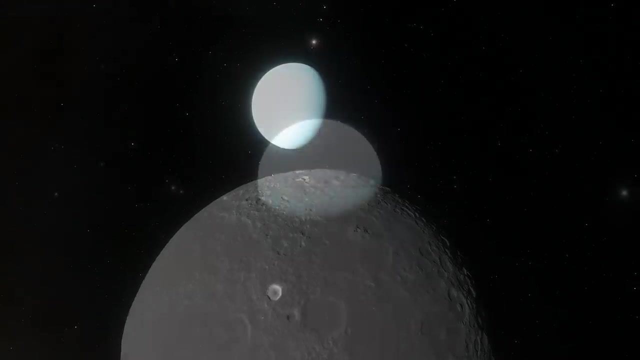 preventing material from spreading out into space. So what might be causing this? Well, as we mentioned earlier, moons play a key role in shaping and maintaining ring systems and, in addition to its rings, Uranus is also home to no less than 27 moons. many 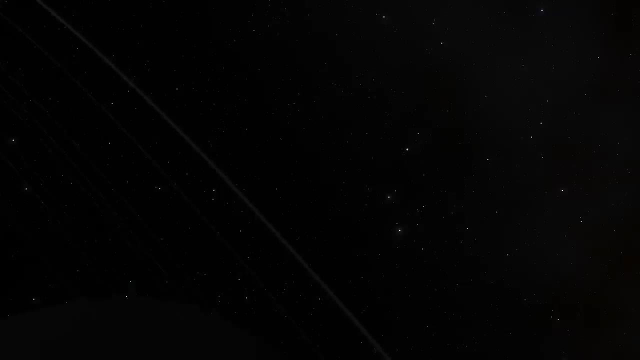 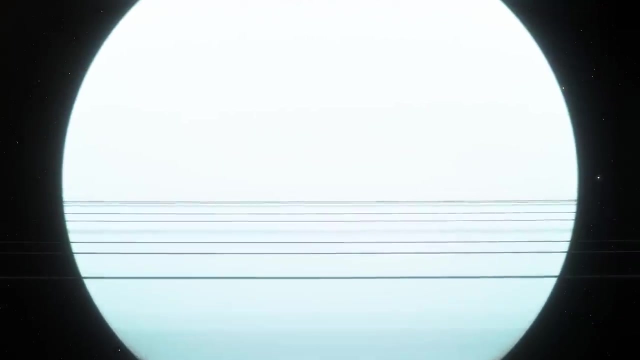 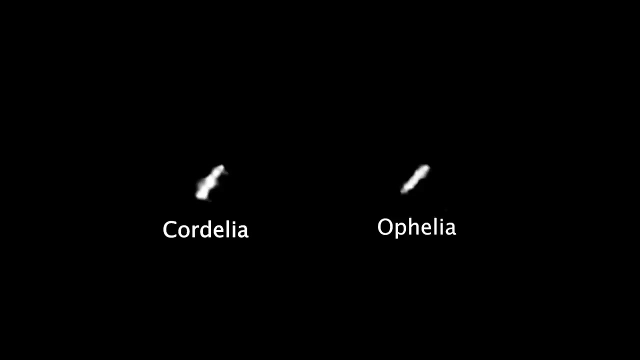 of which are small but orbit within the ring system and exert tidal forces, And this is how we think the rings stay so fine. The Epsilon Ring is circled by two small moons, each around 50 kilometres in diameter- Cordelia and Ophelia. These moons provide like-for-like gravitational kicks and they can be used 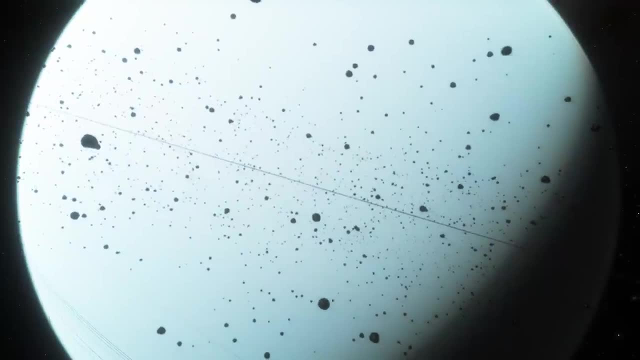 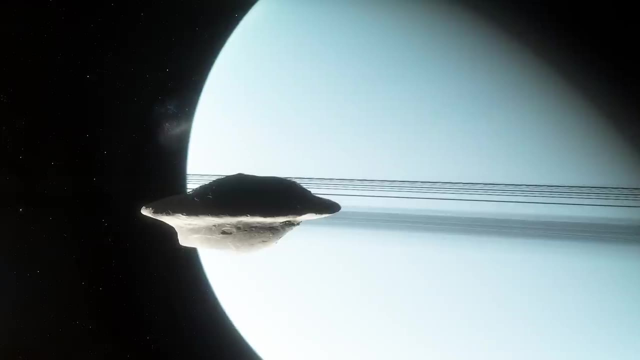 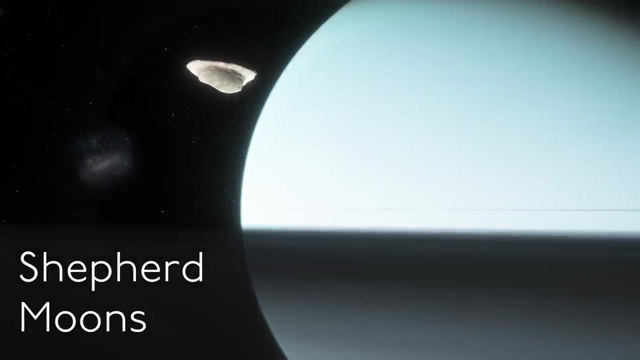 to move around the ringlet and as moonlets within the Epsilon Ring begin to spread out, the two moons pass either side and the balanced gravity of each shepherds the material back into place in the ring. Thus Cordelia and Ophelia are referred to as Shepard Moons- satellites. 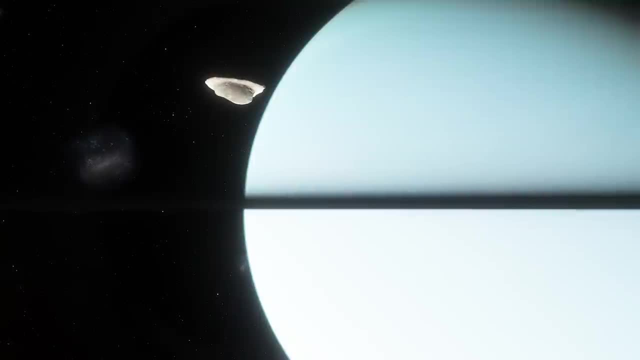 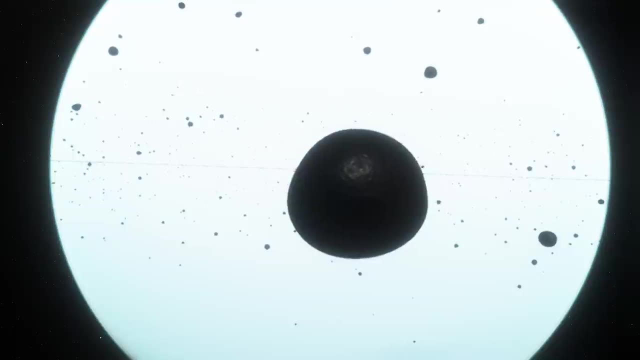 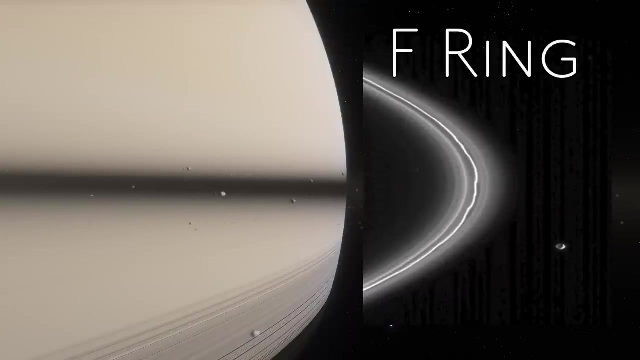 which exert counterbalancing influences on particles within a ring system, neatly preserving the structure in a never-ending game of Moonlet Volleyball. A similar process plays out within Saturn's rings- areas in the F-Ring split, and segment into strands which diverge from one another but are pushed back into place by Saturn's 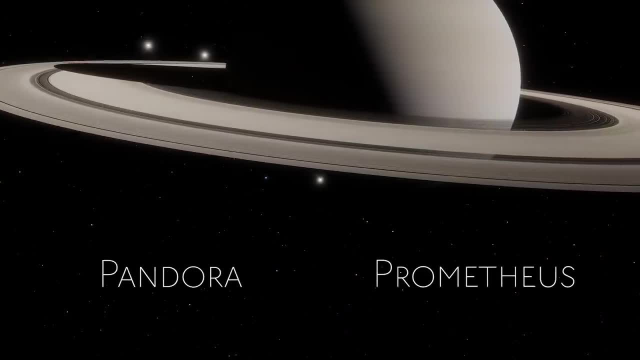 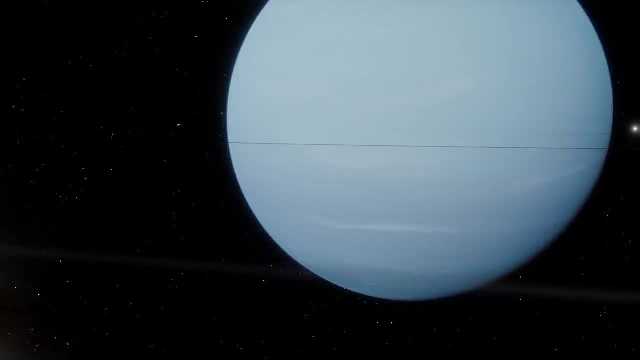 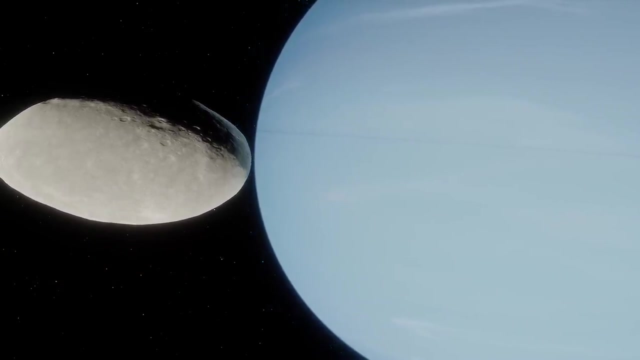 Shepard Moons, Pandora and Prometheus. Neptune also houses a tenuous, dusty ring system which is comprised of narrow ringlets similar to Uranus, implying that it may also have Shepard Moon satellites which keep its rings bound. Unfortunately, though, Shepard Moons, like Cordelia and Ophelia, are incredibly small. 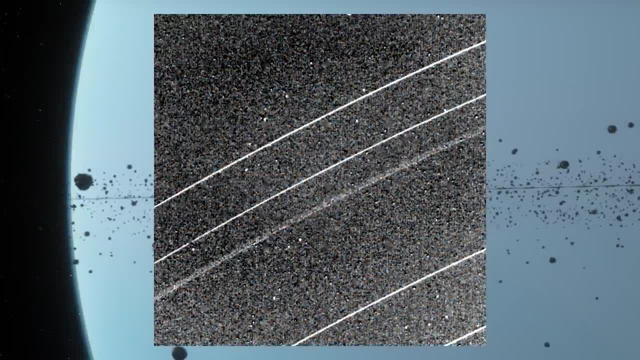 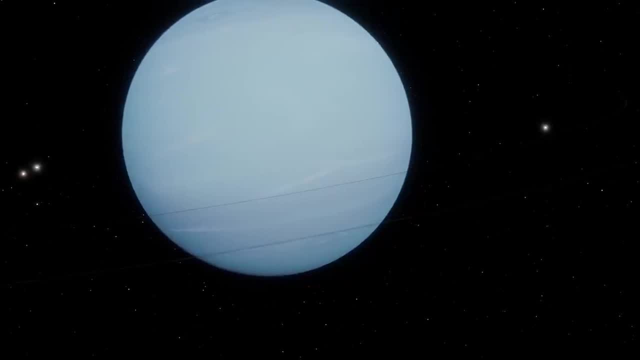 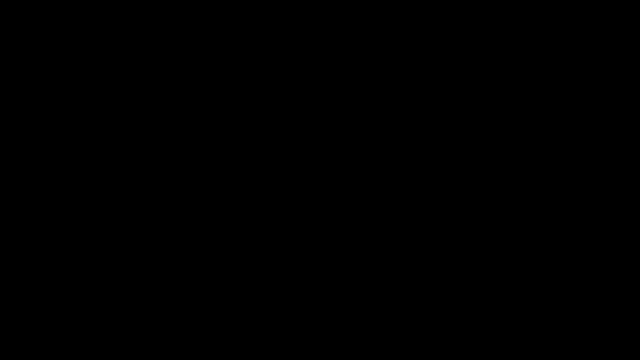 and difficult to identify within a ring system of Moonlets from a passing spacecraft like Voyager, And so it's likely that both ice giants still have undiscovered satellites which shepard their ring systems and keep them in the state that we see today. Alright, time for the big finish, And I mean really big finish. We know that the ring systems 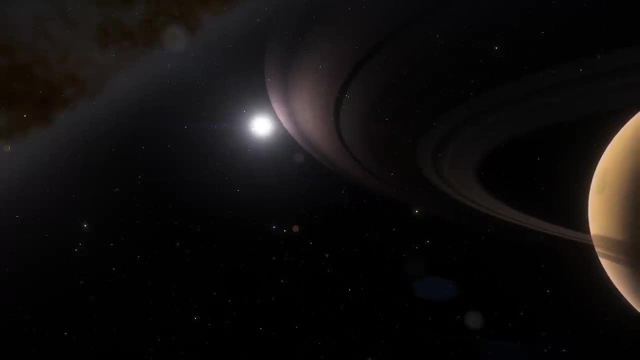 in Saturn have been used to keep the planets in place for centuries and are not only used for the purpose of protecting the planet, but also to protect the planet from the effects of the. know hardly anything about ring systems lying beyond the solar system, but we've managed. 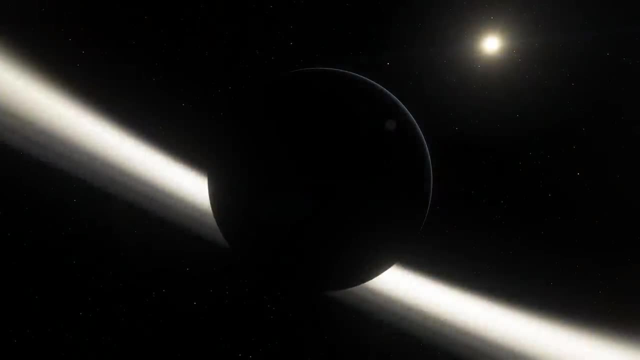 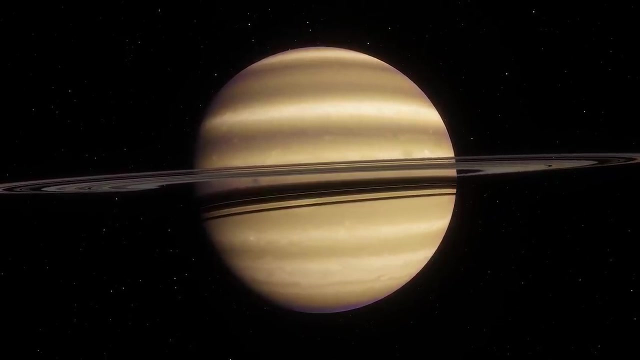 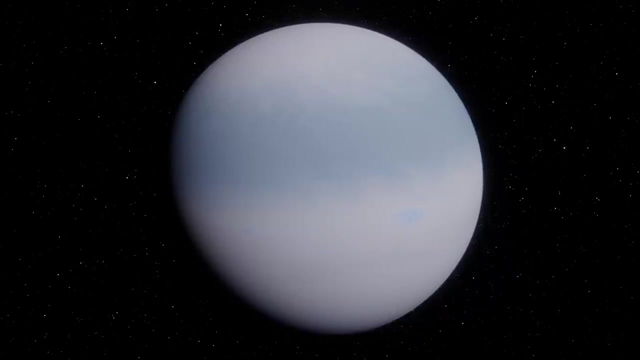 to identify one simply because of its staggering size. It's likely that ring systems are present in other planetary systems like ours, but the problem is we can't see them by looking through a telescope- in fact, we can't even see extrasolar planets that way. Instead, 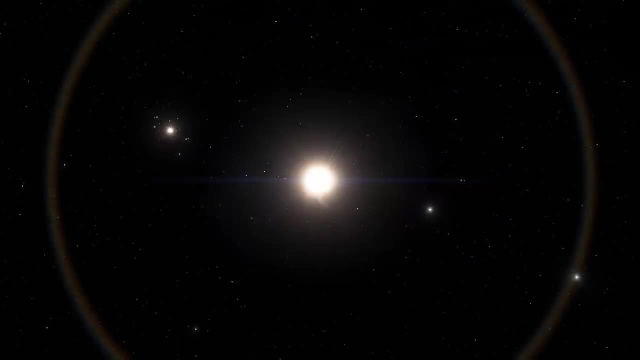 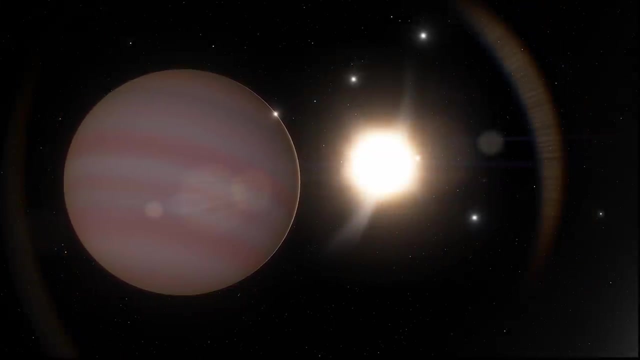 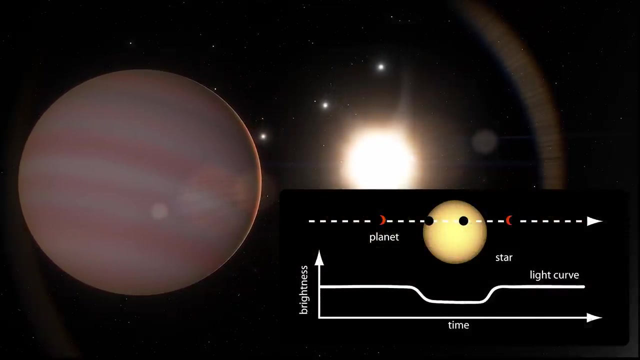 we detect exoplanets by waiting for them to pass in front of their parent star relative to the Earth and block out some of the light. Then we are able to reverse-engineer some of the properties of what's transiting by mapping the light curve of the star. Unfortunately, 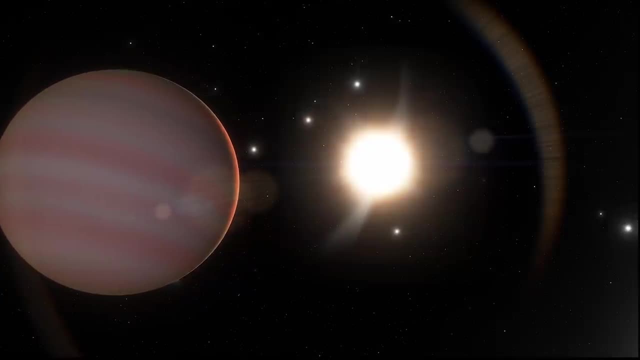 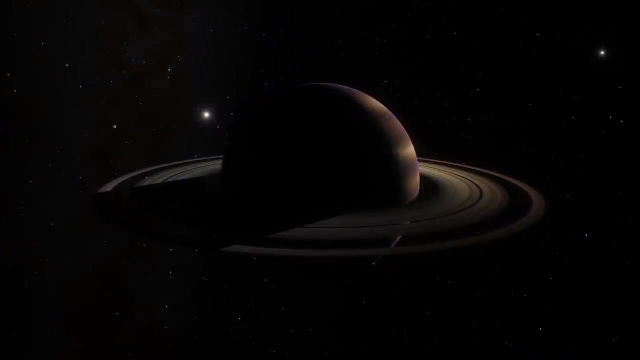 this transit technology is only just about able to identify planets with accuracy- it simply doesn't have the sensitivity to detect the average ring system from so far away. However, we're able to detect exoplanets by waiting for them to pass in front of their parent stars. However, there is one ring system out there that is so large that it was simply unmissable. When an object transits in front of a star and blocks out the light reaching Earth, for planets, we can expect a dip in brightness of a few percent at most. 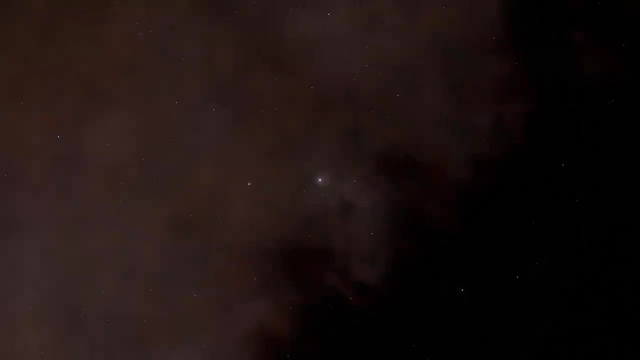 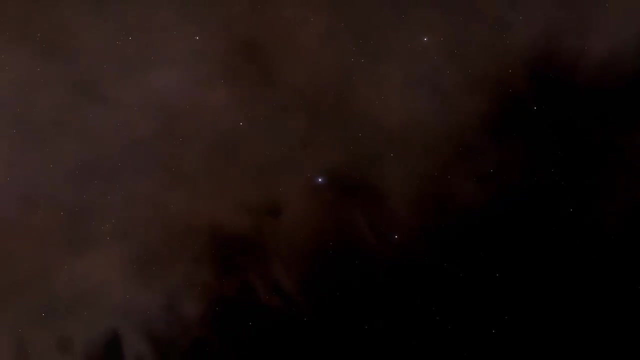 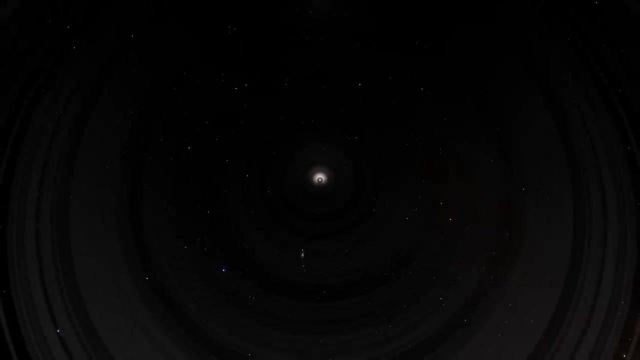 For larger and more obstructive objects such as clouds of dust and gas, up to one fifth of the light can be extinguished, But when we saw a transit which blocked out the light curve of a parent star, it left us scratching our heads. 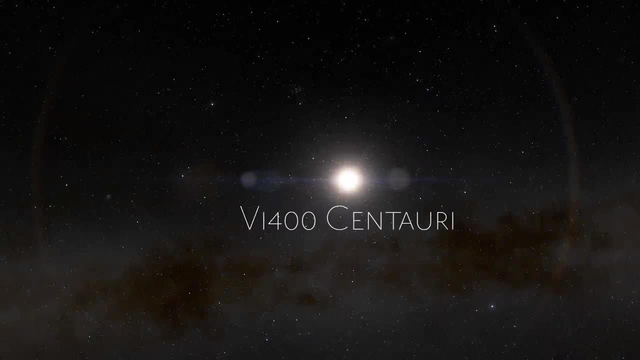 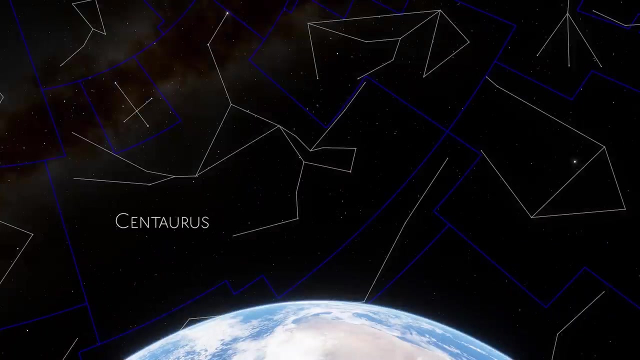 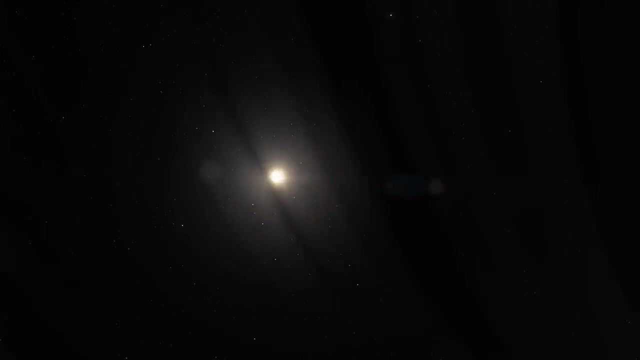 First noted in 2007,. V1400 Centauri is a young star system around 400 light-years away from the Earth, within the constellation of Centaurus, And while the system was under observation, scientists recorded an eclipse event of the parent star which lasted for some 56 days. 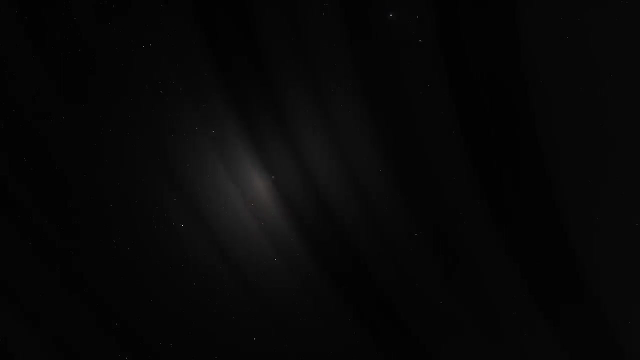 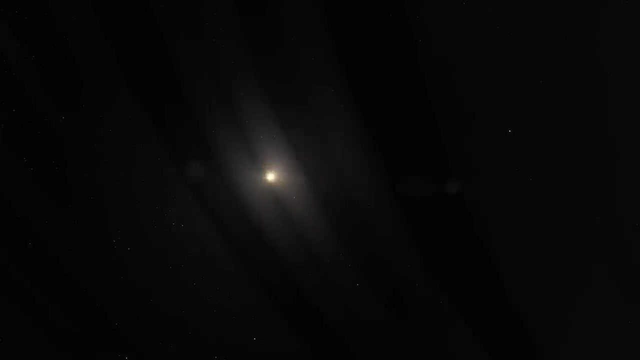 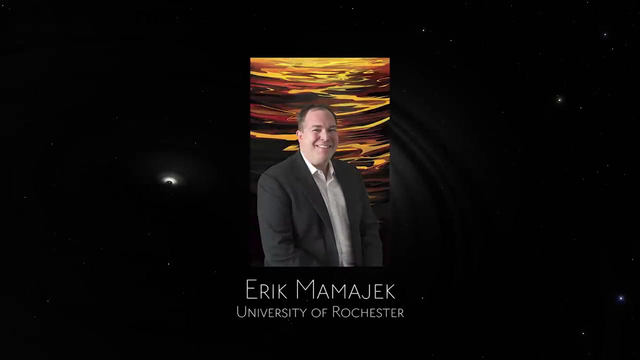 Sometimes the star's light was almost entirely extinguished, But other times light was able to penetrate through clear and definite gaps in whatever was transiting. In 2012,, a team led by astronomer Erik Mamacek proposed that the transiting object also 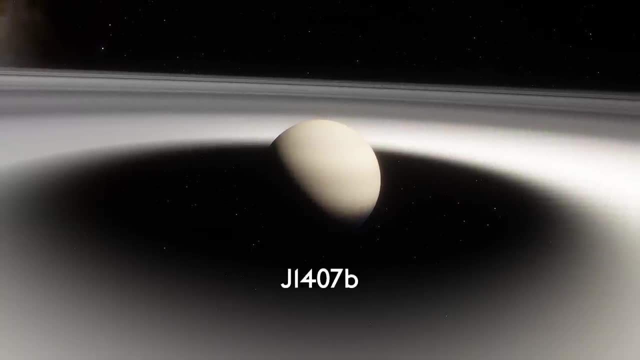 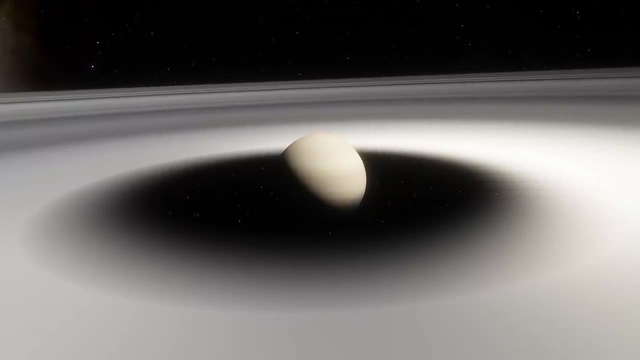 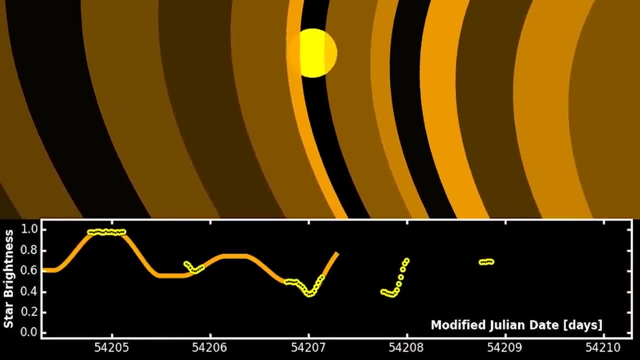 known as J1407b, is a large and massive gas giant, or brown dwarf, surrounded by a ring system of epic proportions. In 2015,, new analysis and research allowed astronomers to model the system, revealing over 30 nearly opaque rings each millions of kilometers wide. The whole system is an 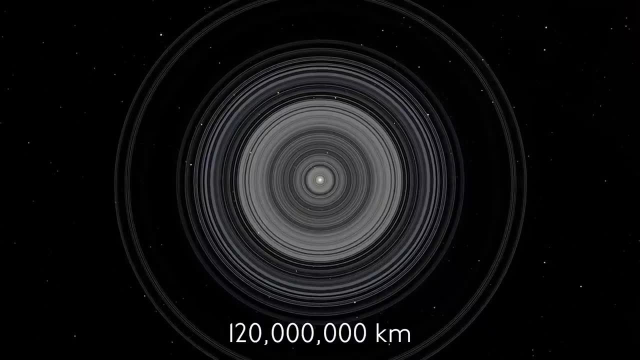 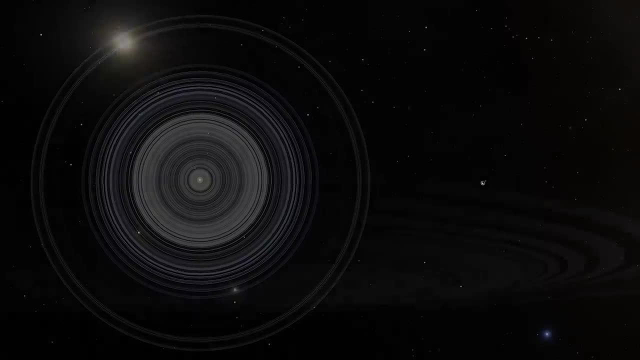 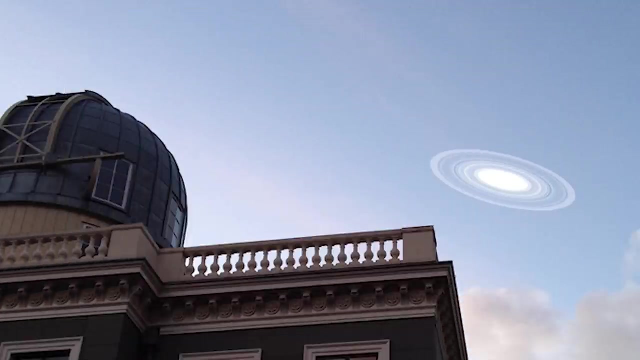 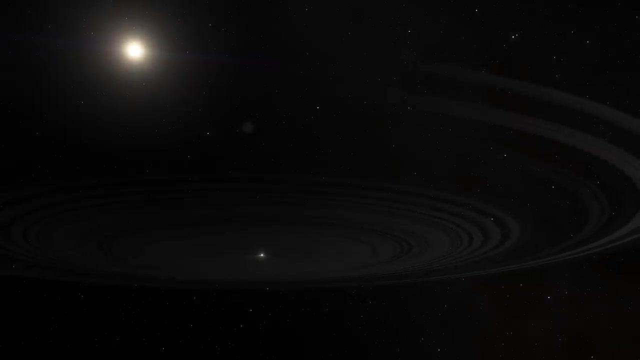 incredible 120 million kilometers in diameter- more than 200 times the diameter of Saturn's icy rings. If J1407b were to replace Saturn in the solar system, then its rings would dominate the night and daytime sky like so. At this size, it's very unlikely that the rings were formed by the break-up of a moon-. 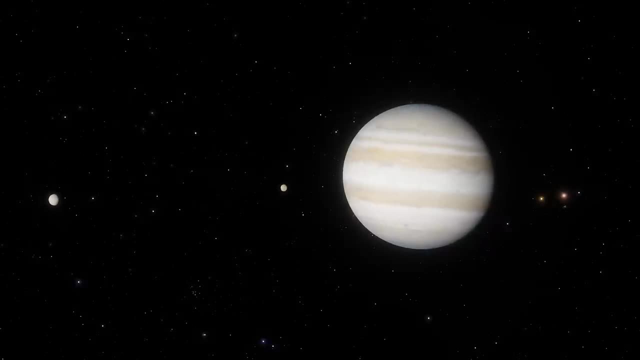 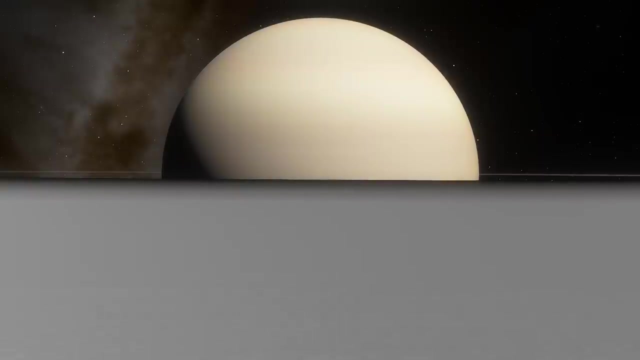 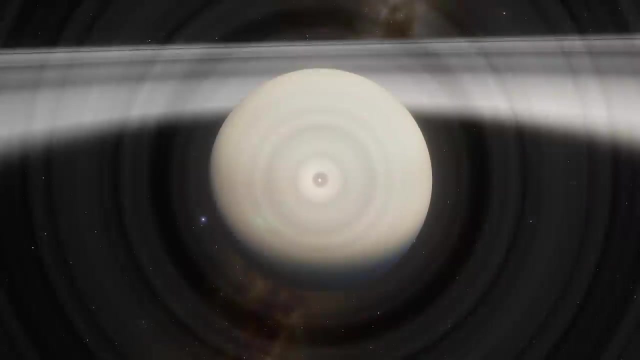 you'd need to grind up all of Jupiter and Saturn's large moons, and then some, to create this much material. Rather, this ring system has probably formed via the other hypothesis we mentioned- they are primordial in origin. J1407b is a young gas giant, but it's not. 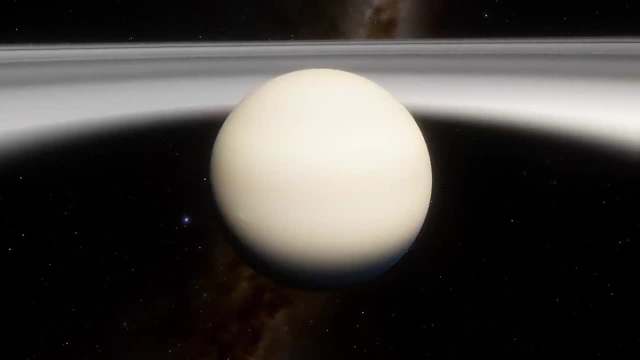 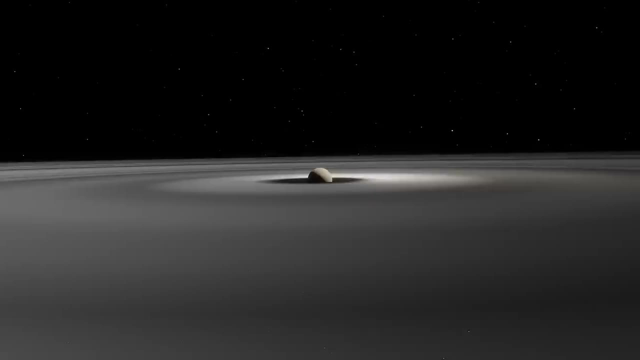 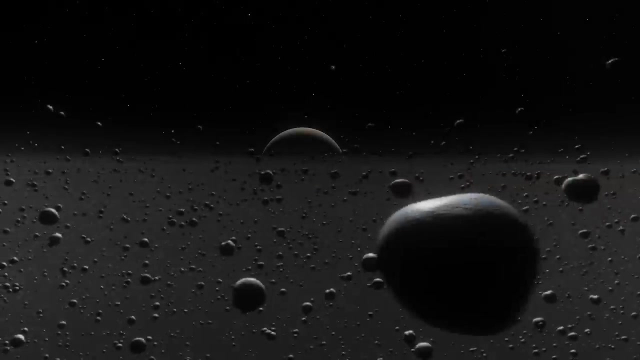 a gas-genius in the final stages of planetary formation- and these rings may not actually be traditional rings, but rather a planetary disk from within which the gas giant has formed. The material in these rings consists mostly of protoplanetary dust and will lay the foundation. 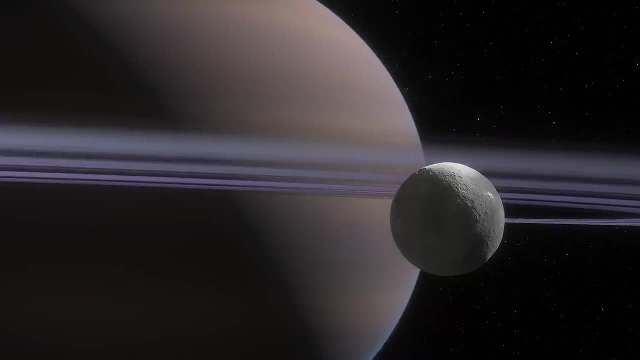 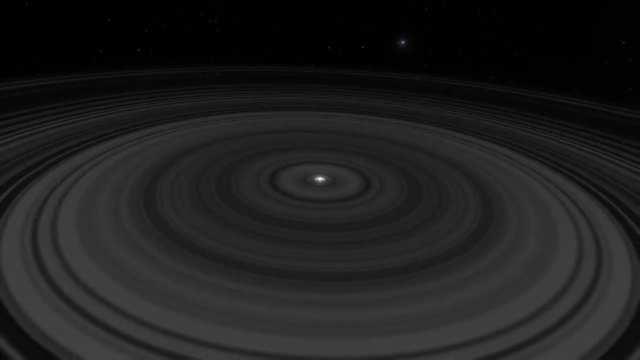 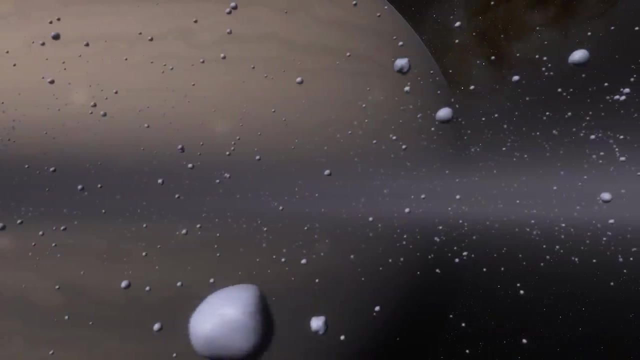 for co-accretion- the birthing of new natural satellites. Because of its enormous scale, vast majority of this material lies well outside the planet's Roche limit, and so it will be able to accrete into larger bodies, and we believe that this is already happening, Even though 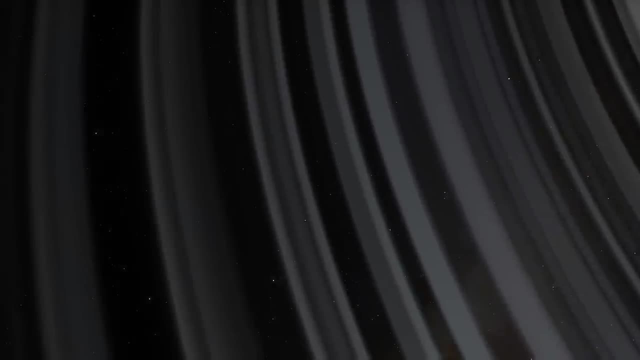 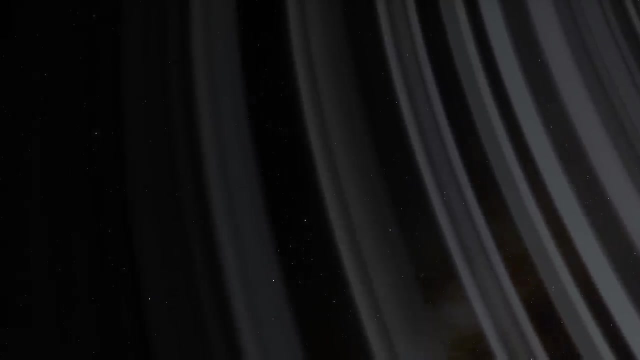 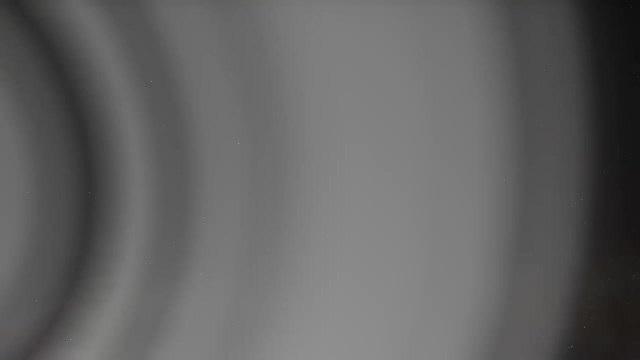 J1407b's eclipse event lasted for weeks. astronomers noticed variations in the star's light curve as frequently as on hourly timescales, owing to fine structures which are forming inside. In addition, astronomers have noted a definite gap in the ring system around 0.4 astronomical. 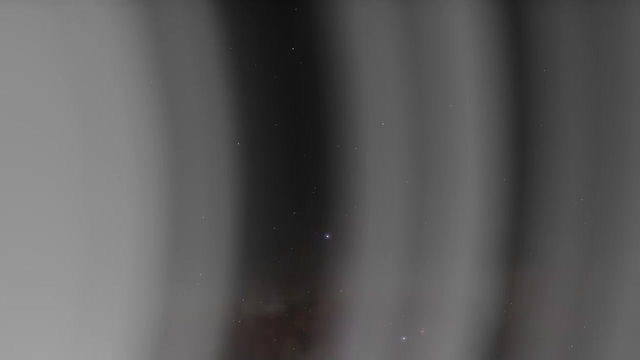 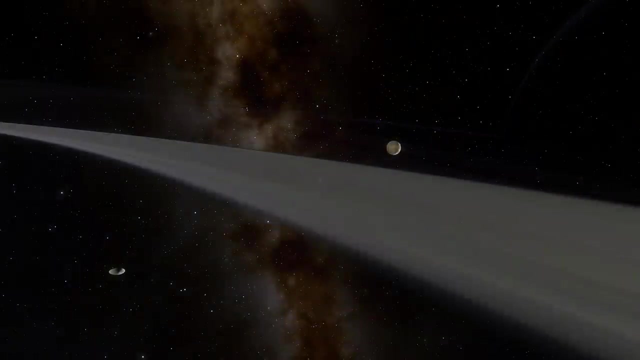 units away from the planet, where we think that an exomoon has formed and cleared a trail in the dust And over the next few million years, the majority of this material will condense into large and complex satellites like Europa, Enceladus, Titan and Ganymede. The planet J1407b is known as a surface-to-surface satellite and is known as a surface-to-surface satellite. The planet J1407b is known as a surface-to-surface satellite and is known as a surface-to-surface satellite. 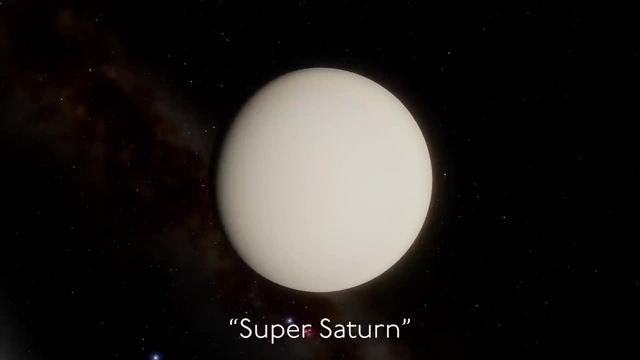 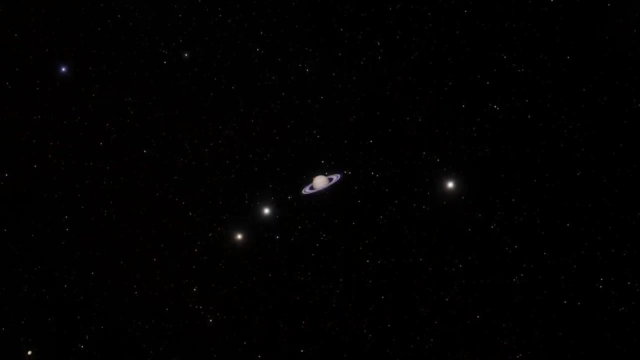 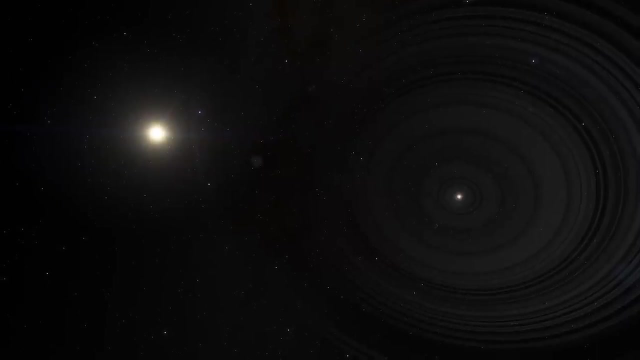 And it boasts a lot of potential for a rich subsystem of moons on a scale much greater than the ones we see around the gas giants today. But we have caught this system in its fledgling stages. It'll be millions of years before these new moons form, and so we probably won't be around. 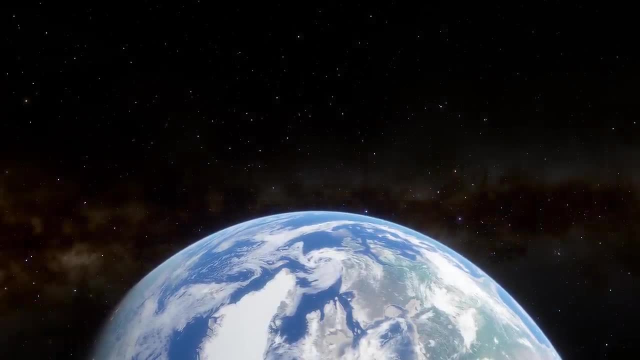 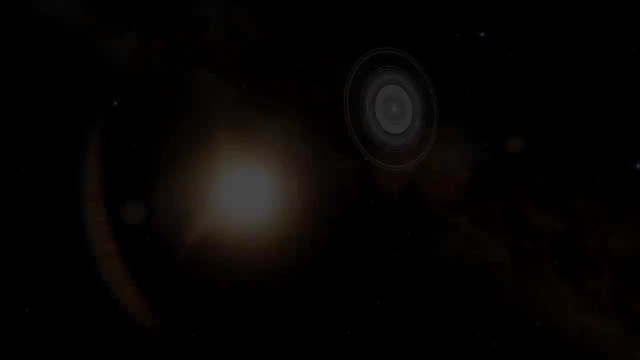 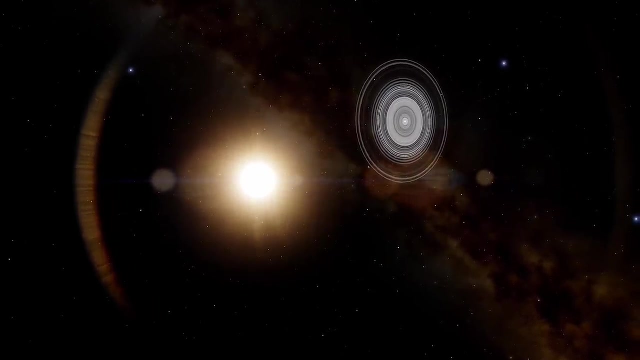 to see it unfold, A reminder of the enormous timescales we're dealing with when waiting for things to happen in space. But hey, at least we've got something pretty spectacular to observe in its place in the meantime, Perhaps when the James Webb telescope finally launches. 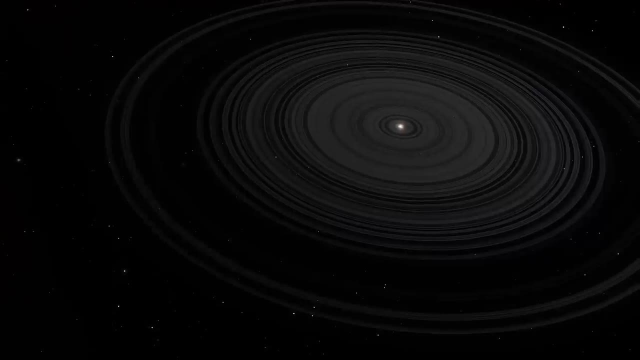 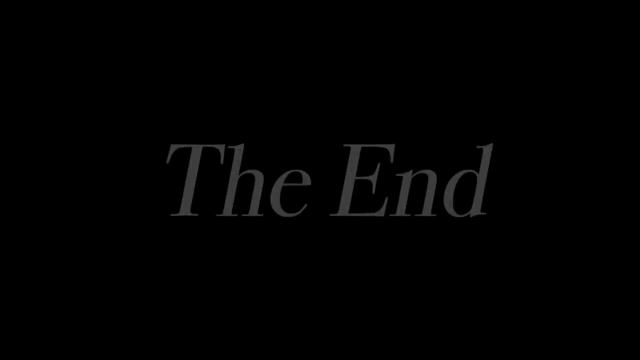 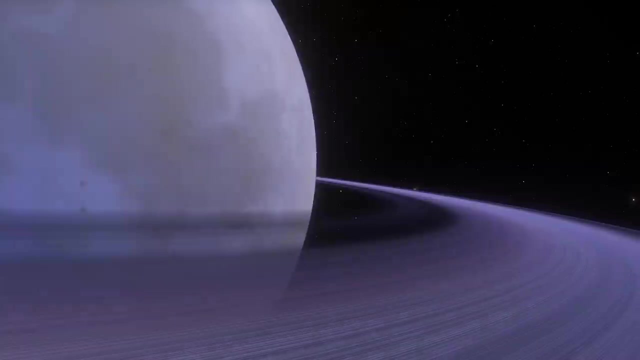 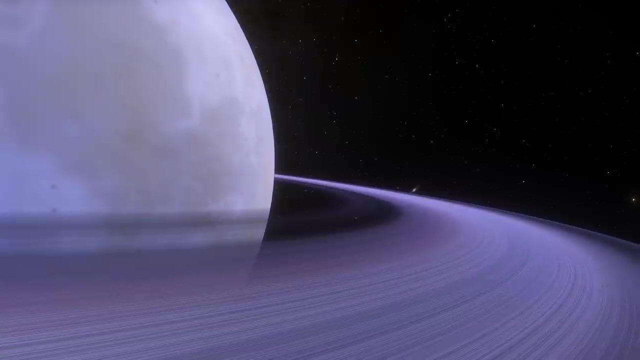 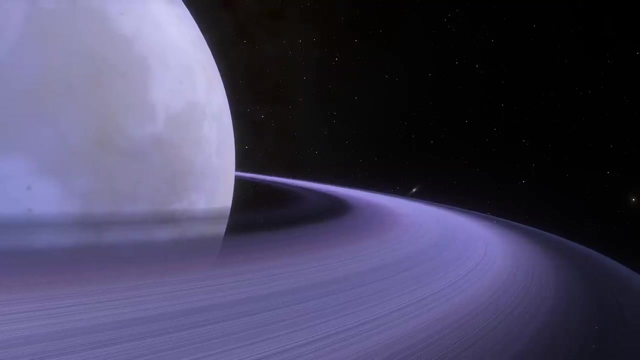 its unparalleled sensitivity and detail will help us to peer deeper into this unique system. NASA Jet Propulsion Laboratory, California Institute of Technology.